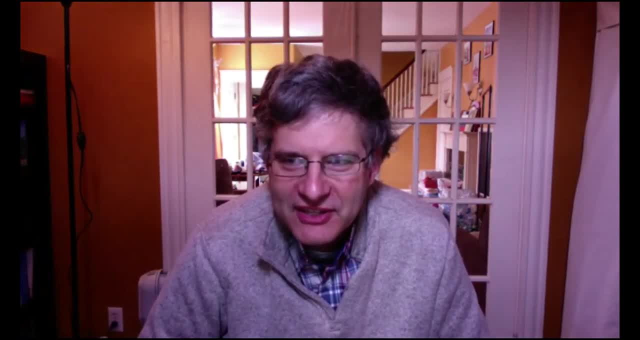 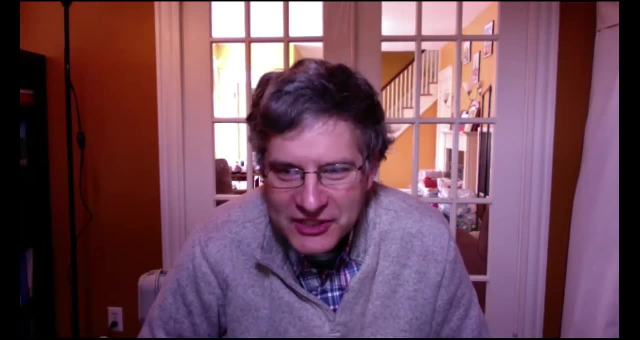 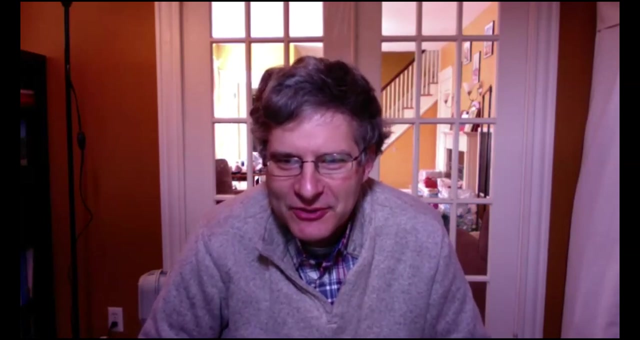 becoming a graduate student in our department And he is scheduled to defend his PhD this summer and start a prestigious Dirac Postdoctoral Fellowship in August Now. Ken was a truly outstanding student, one of the very, very best I saw in our department since I joined. 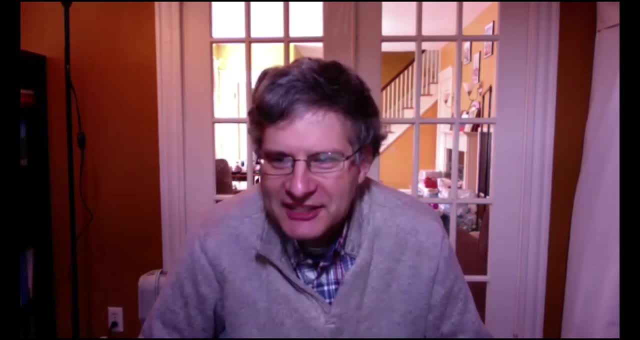 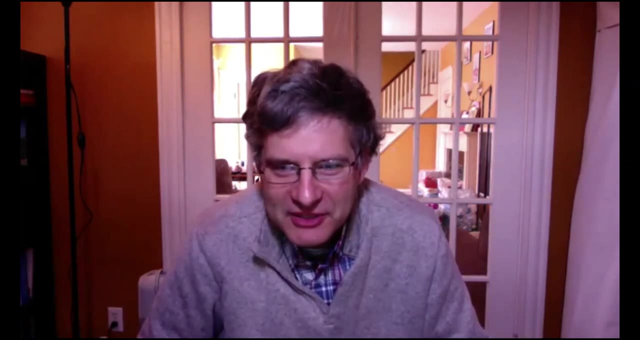 it in 2003.. So this was recognized by an number of awards, Of course, this Galking Fellowship, as well as the full membership and Sigma 3.. And I should mention that Ken Ken has been an outstanding teacher both in Hong Kong and at Brown and won multiple teaching awards. 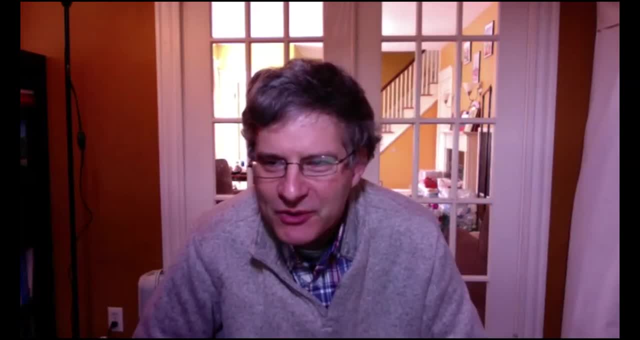 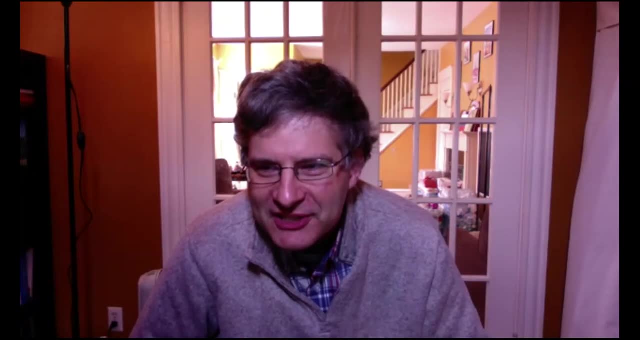 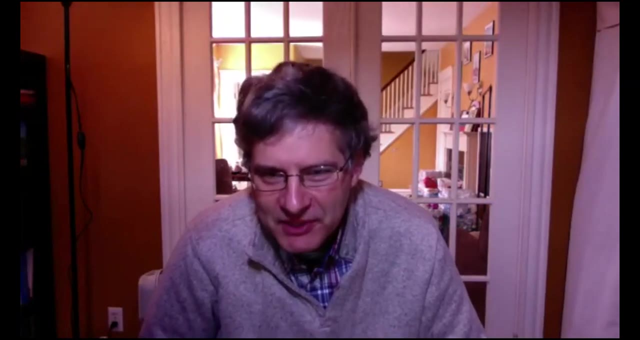 But he is an even more outstanding researcher, someone who is truly very knowledgeable, very creative, very bright. So I should mention, even though he didn't get his PhD yet, he is already an author of seven papers on a very broad range of topics, from optics to mathematical physics. 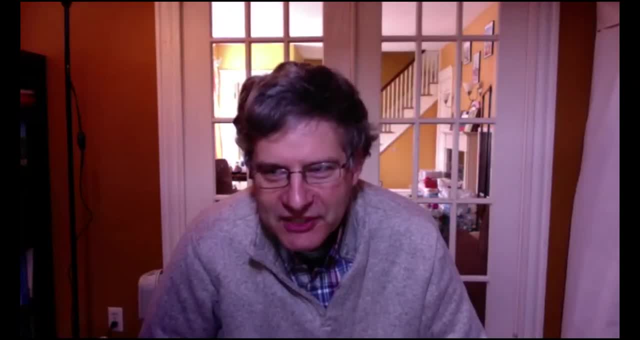 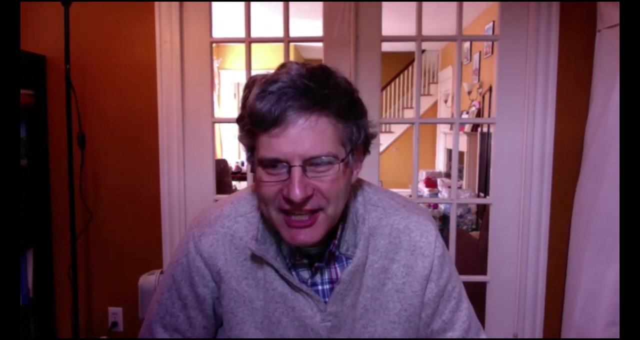 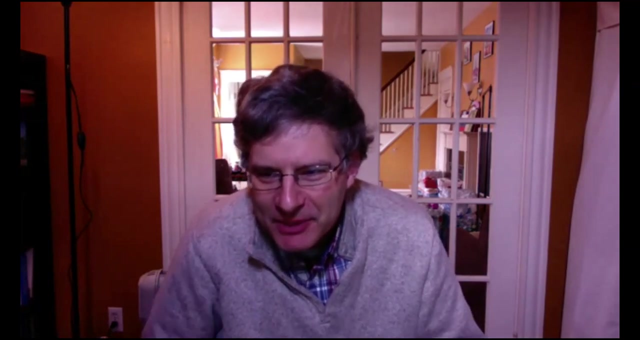 And, what's perhaps more important, two of those seven papers are without co-authors. So we always want our students to become completely intellectually independent, but in practice it's a very, very tall order for someone who is at that PhD stage And it's just very hard to develop your own research direction. pose a question, solve that question, write a paper, do everything on your own. 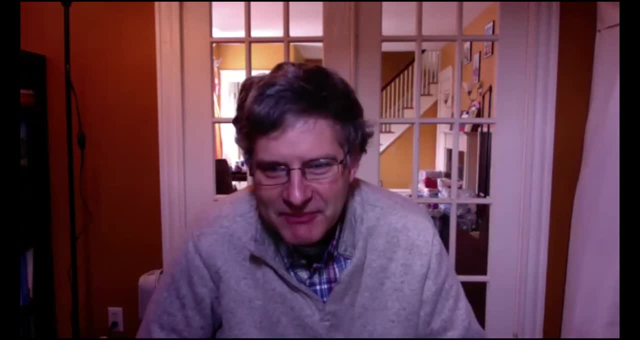 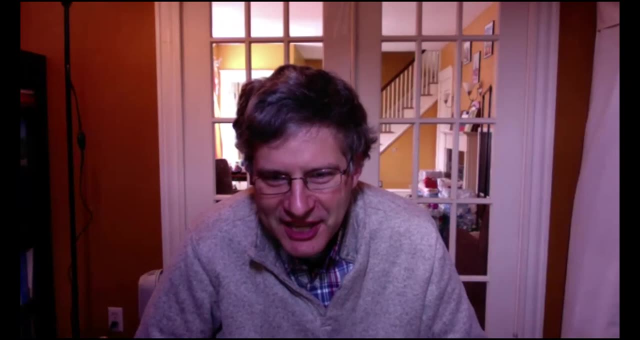 So very few PhD students can do that. We normally expect that people would develop the skills already as postdocs, and Ken did that already twice. So he is really an outstanding student, really a student with whom it's a great pleasure to work. 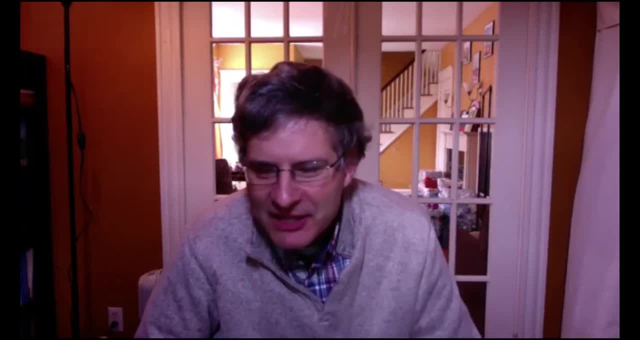 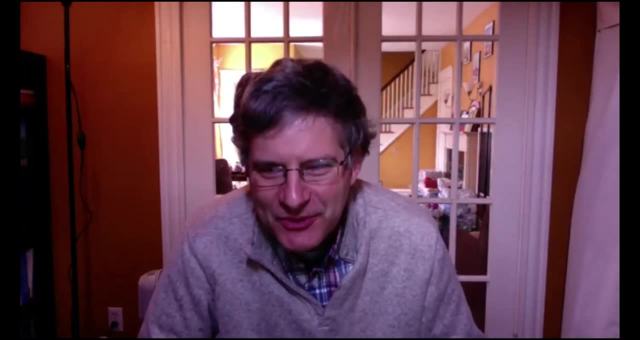 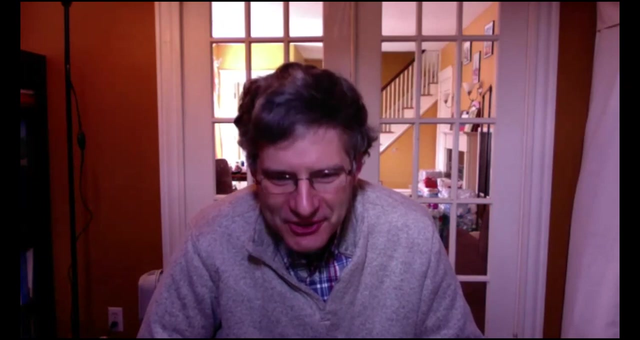 And it goes without saying that he is exceptionally, exceptionally knowledgeable in physics and mathematics. But perhaps because that's a rather special event, I would mention something else that we don't normally mention in our formal introductions, Because Ken is not just a great physicist, he is a true intellectual. 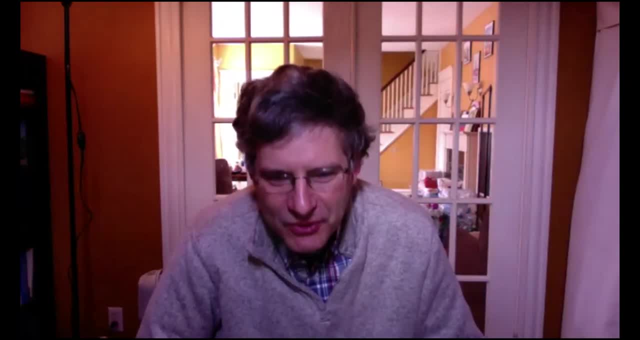 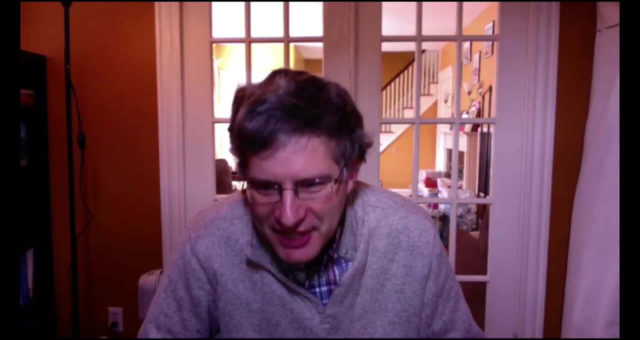 And I really never met a student who would be so knowledgeable about so many things. For example, he is a great expert on philosophy, Western and Eastern, And another thing. so I never met a person who would know better ancient and medieval Chinese classics. 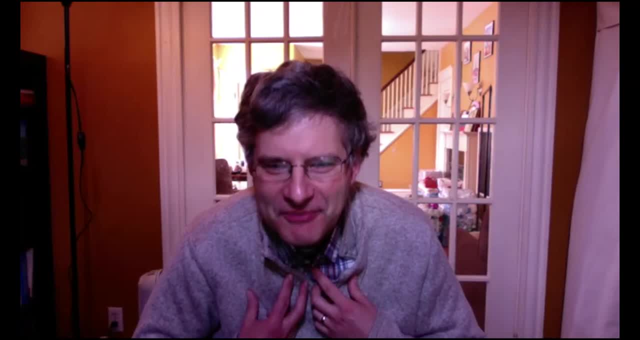 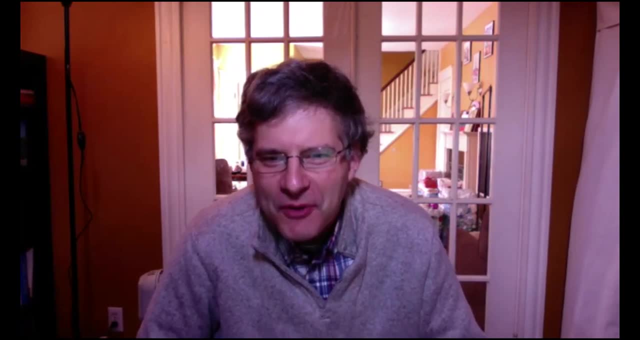 So I always learn from my students as much as they learn from me. But that's physics, mathematics, occasionally chemistry. I think in the case of Ken, I learned more from him than he learned from me, because physics and mathematics is always an exchange between the advisor and the student. 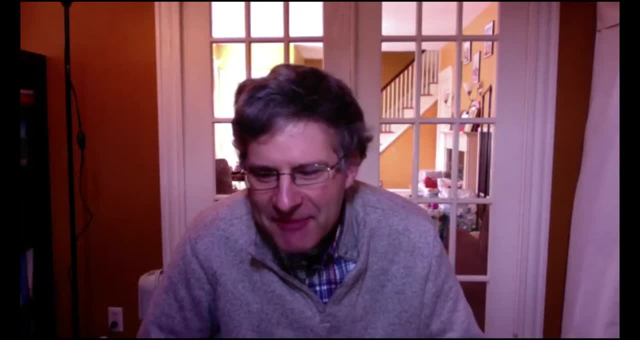 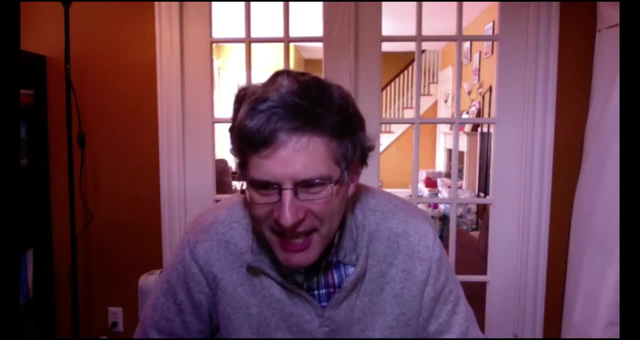 But there are very many other things to learn from him. So I am really proud that we have such an outstanding student who is a recipient of our Galkin Award this year, And now this Galkin presentation actually posed a very unusual challenge. 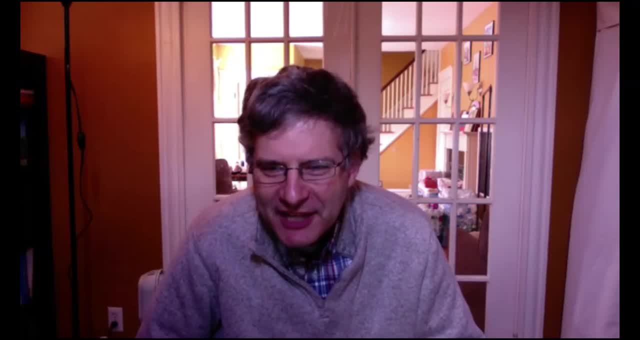 Because Ken worked on so many topics, it was very hard to decide what to tell about. There is no way to speak about all he did at Brown. Eventually, Ken decided to speak on his work about the 16-fold way, And I think now it's time for him to start. 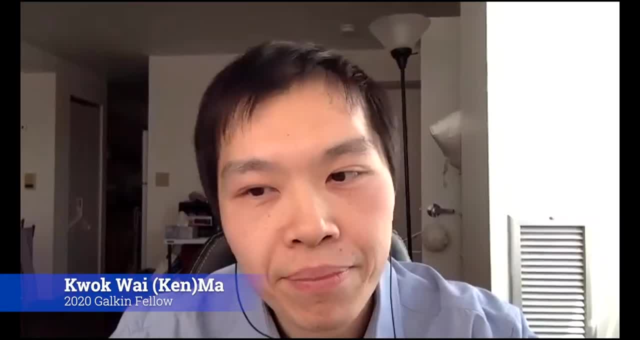 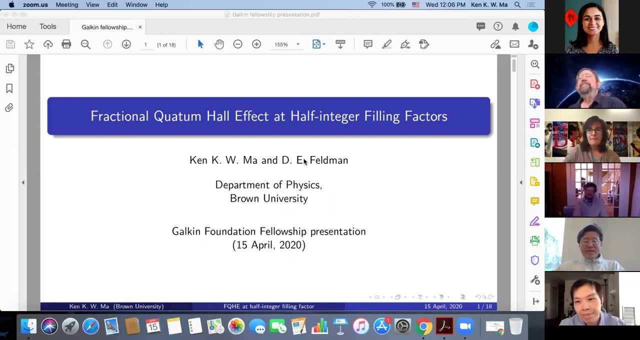 Thanks a lot, Dima, So let me share my screen, Okay, so can all of you see my PowerPoint now? Okay, so first of all, I need to thank Dima for such a nice introduction, And I also need to thank the organizers for inviting me to give a talk here. 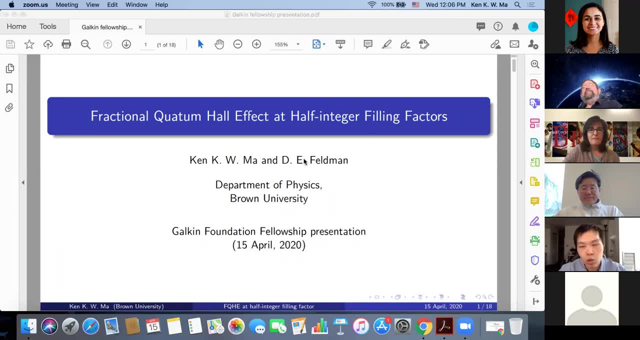 So today I will talk about fractional quantum point effect at half-imager viewing factors. This is a research that I collaborated with my advisor, Dima Feldman, So at this moment, if you don't understand what the title is, that's okay. 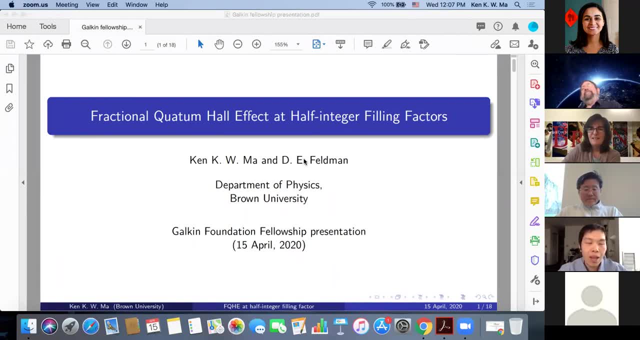 And I hope you understand it more after my talk. Okay, so one of the interesting things, as you will see later, is that at half-imager viewing factors, there are many possible candidates being proposed to describe the fractional quantum state, In particular, at the viewing factor of 5 over 2,. there is always a disagreement between the candidates, supporters and students. There is always a disagreement between the candidates, supporters and students. There is always a disagreement between the candidates, supporters and students, And there is always one next to nothing, which is what they are explaining to you, And one of the things that comes to mind is this idea that the material is always supposed to beChat-t spider. 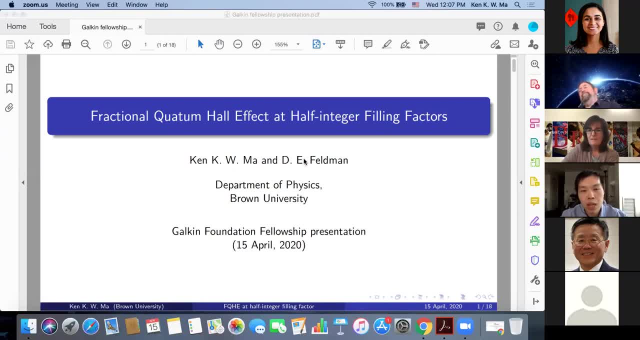 And there was a piece of research that was done in the 1980s, which was a very interesting idea, And this is based on the theory- the theory of location that was held in the early 1980s- that we can find the point of view of the information, that the data was obtained. 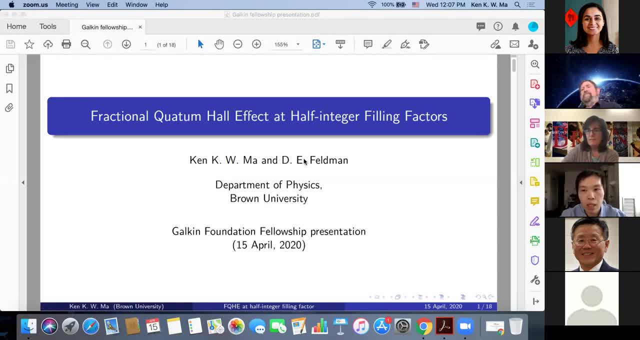 being the same from the numerical simulation and experimental data. But we know that physics is an experimental subject, so the later of the fractional quantum state can only be revealed from experiments. So in today's talk I will do two things. First I will introduce what is half-imager fractional quantum state. 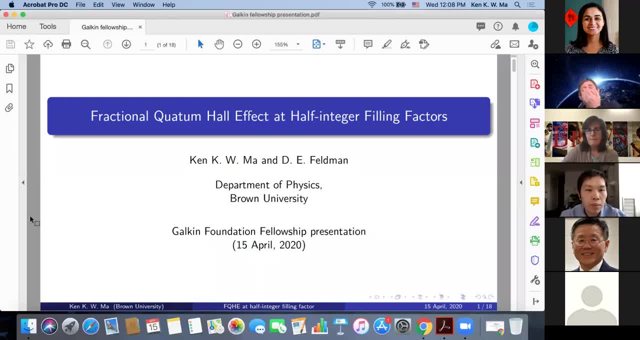 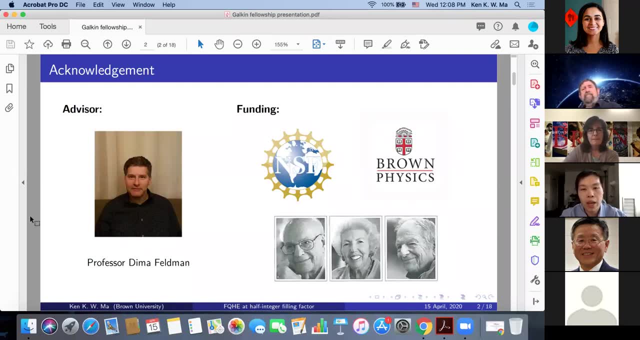 of doing factors Okay. so first of all, I must thank my advisor, Professor Timmer Feldman, for his guidance and support. I also need to thank different funding agencies, including NSF Department of Physics and, of course, the Galkin Foundation, which brings me to today's talk. 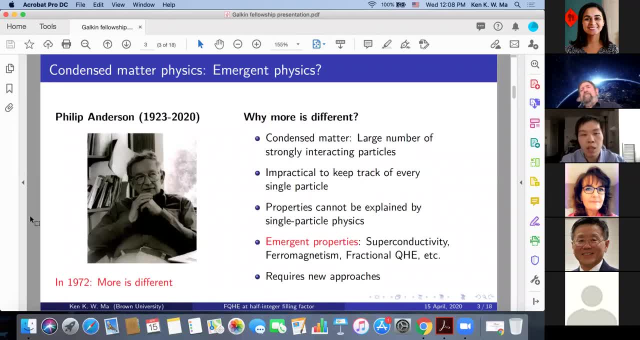 So let me start by quickly reviewing what is condensed metaphysics and what a condensed metaphysicist does. So I think one of the best summaries comes from Philip Anderson. In 1972, Anderson wrote a famous paper with the title More is Different. Nowadays, this sentence is commonly used. 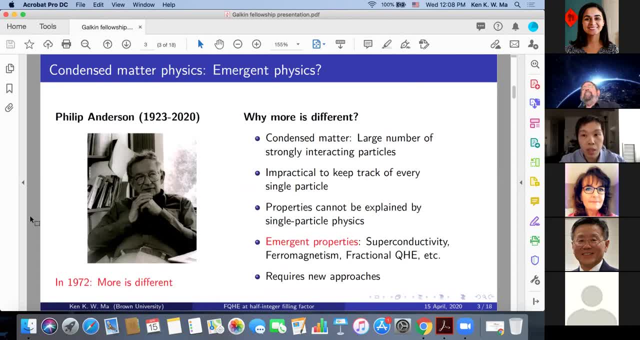 as a motto of condensed metaphysics. So let me discuss why more is different. So in a condensed metal system, there is a huge number of strongly interacting particles. These particles can be electrons, ions, etc. Now, in principle, we may write down an. 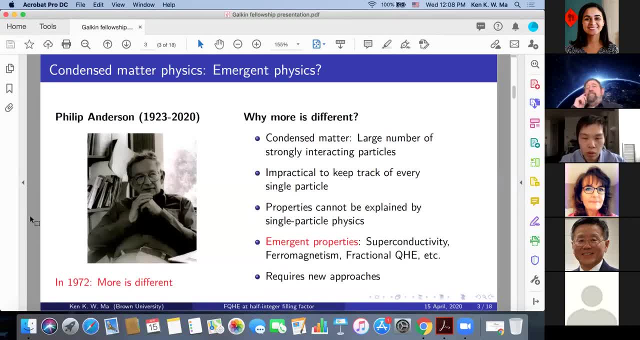 equation to describe the motion of a condensed metaphysics, The motion of each particle. But given such a large number of them and their strong interaction, this task becomes impractical. At the same time, the strong interaction between these particles will lead to some emergent properties which cannot be explained. 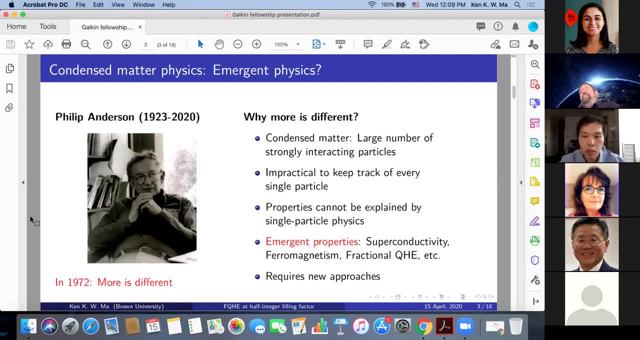 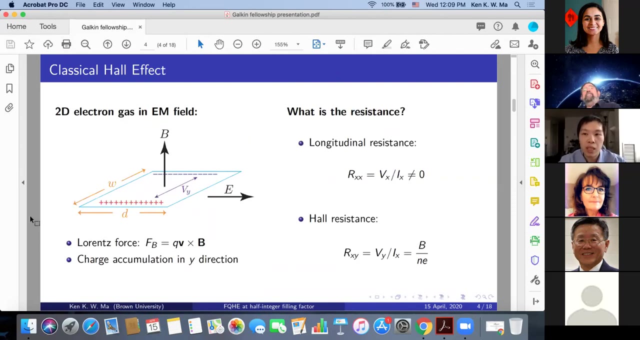 from single particle physics. Some famous examples include superconductivity, global magnetism and- the main character today, fractional quantum point effect. In order for us to describe this emergent phenomena, condensed metaphysicists need to develop new approaches. So, before going to quantum point effects, let me quickly reveal what is. 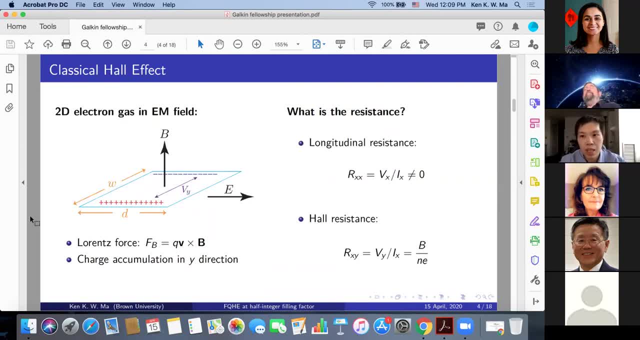 classical point effect. Suppose I have a conducting material and place it in an electric field, then charges will move and generate an electric current. Now I apply a permanent magnetic field to my sample as below: moving charges will experience a low-end force in the magnetic field. 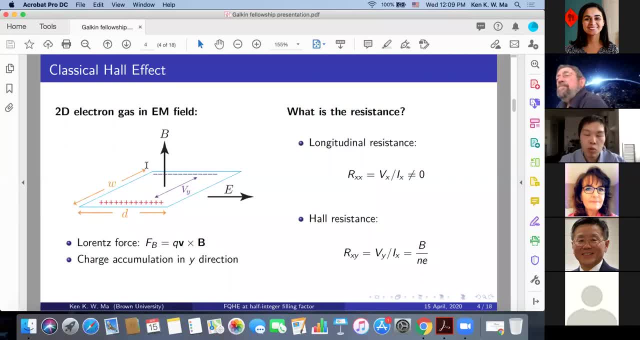 So let's say that the current is a constant force and the electric field is a constant force. Negative charges and positive charges will drift to two opposite sides of the sample, as shown here, And this accumulation of charges will generate a potential in a perpendicular direction to my applied electric field. 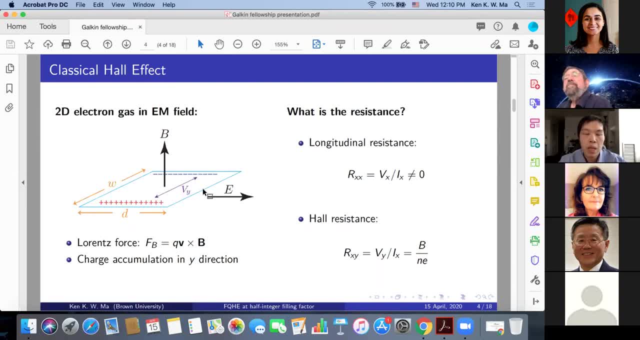 And we call this potential as all potential. Now, if I look at the resistance of my sample, I have two different terms. The first term is the longitudinal resistance that we usually measure. It is given by the ratio between the potential difference given by the electric field and the electric current. 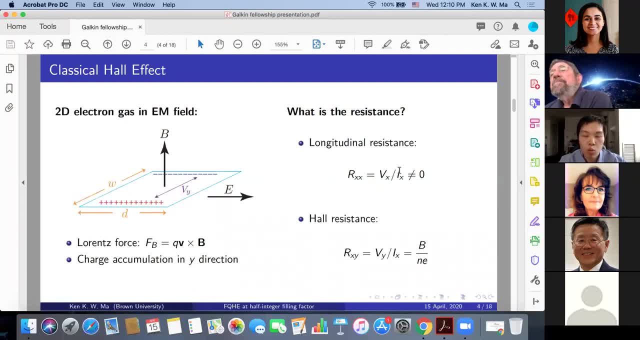 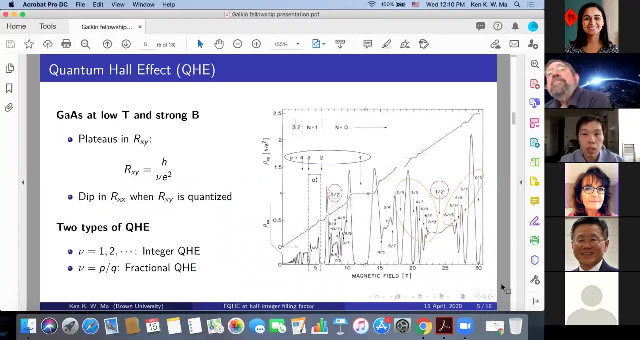 The second term is the Hall resistance, which is defined as the ratio between the Hall potential and the electric current, And this Hall resistance should scale linearly with the magnetic field. So what happens if we perform a similar experiment in two-dimensional electronic system, let's say two-dimensional electron gas in semiconductors? 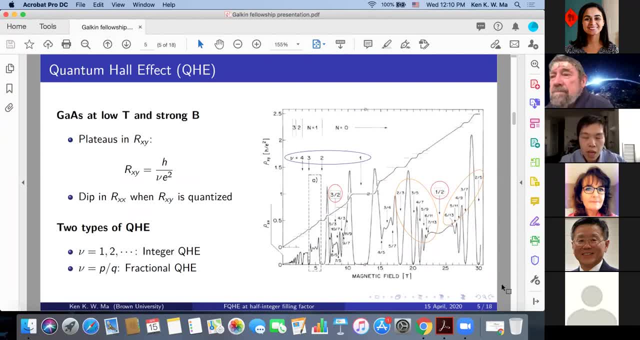 and cool it down to low temperature, let's say several Kelvin, and pay it under a strong magnetic field, let's say around 5 to 15 Tesla. Here I show you some experimental data which was obtained about 30 years ago. As you see here, instead of just a single straight line against magnetic field in the Hall resistance 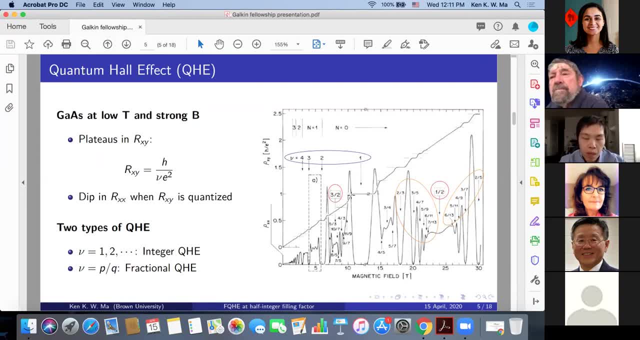 we also see some steps or petrodes in the Hall resistance. At this petrodes, the Hall resistance is so precisely quantized to a combination of fundamental constant, that is, H, the Planck constant, E squared, the electron charge squared, and 1 over a coefficient mu. 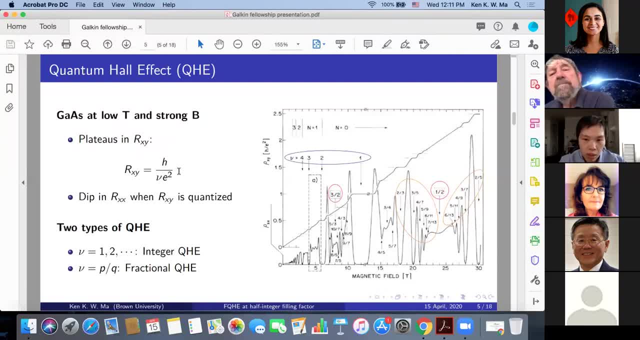 I will discuss this mu in more detail Also. at the same time, at the position where we find those petrodes in the Hall resistance, we also find minima and dips in the long-to-tunnel resistance. These two features define a quantum Hall state. 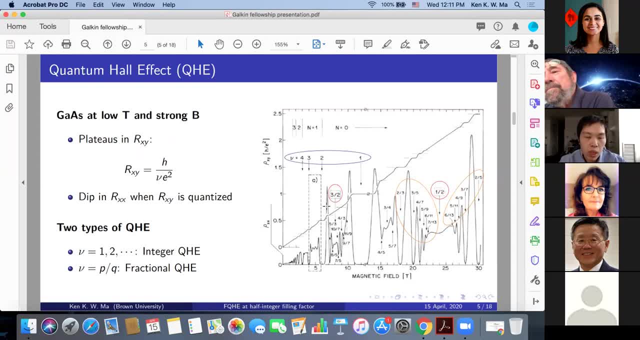 Now let us look at the petrodes more carefully. We see that mu may be an integer. In this case we say: the system is in the integer quantum Hall state. The second possibility is that mu can be a fraction. In this case we call: we have a fractional quantum Hall state. 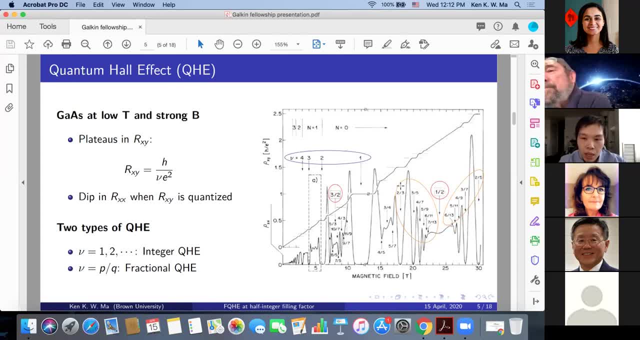 Now let us look at the fraction more carefully. We see that most of the fractions have odd denominators. At the same time, we don't see any petrodes at a given factor- 1-half or 3-half. These two features will be understood later when I discuss the theory of composites. 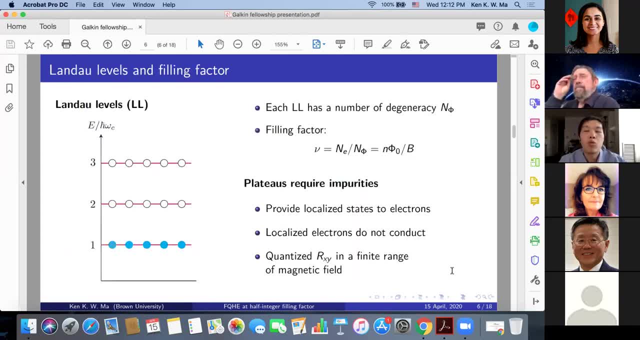 So, generally speaking, it's such a simple matter. It is inspire, which we can use, the Poisson idea behind construction that that quantum. Now consider the situation that I have an electron moving on a two dimensional plane and then I apply a Permedictgeb tycker to it. 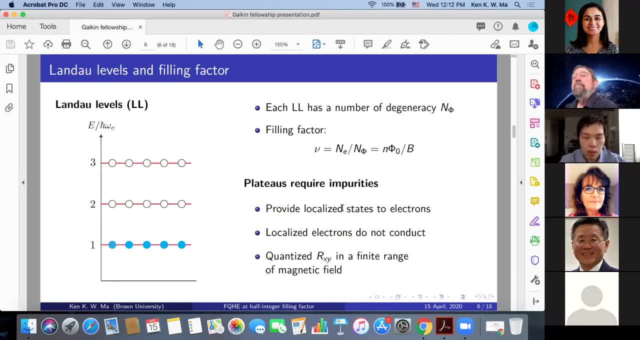 According to quantum mechanics, the energy levels of the electrons would be quantized into something called Landau levels And for each Landau level it can accommodate more than one electron. Suppose each Landau level can accommodate by electrons, as shown here, my system have five electrons, then we can define a fueling factor. i mean the fueling factor is: 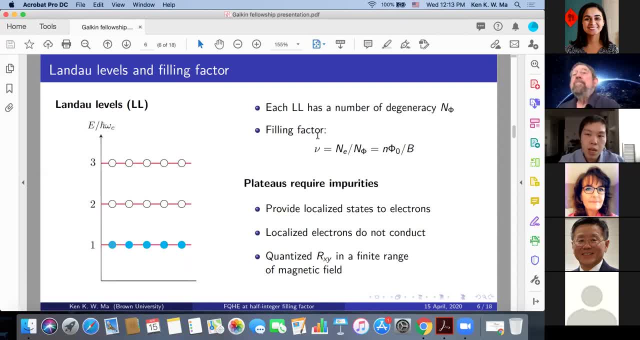 defined as the ratio between the number of electrons i have in my system and the number of electrons that can be accommodated by each landau level. in the situation here, i have five electrons and each landau level can accommodate five electrons. then i will have mu equals to one. 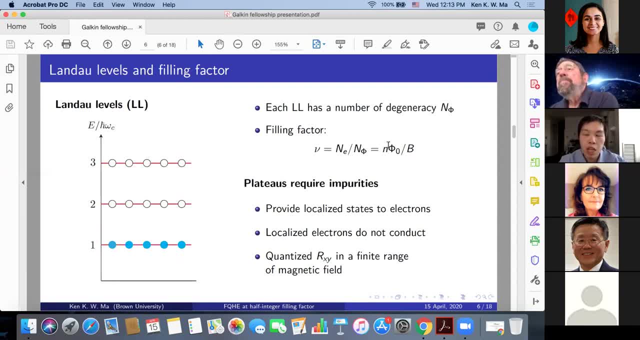 in general, this ruling factor depends on the number of electrons per unit area and the magnetic field that i apply, so in an experiment i can change either one of them to reach the value of mu. okay, so suppose a landau level is completely filled, as shown here now, as shown in the figure, we 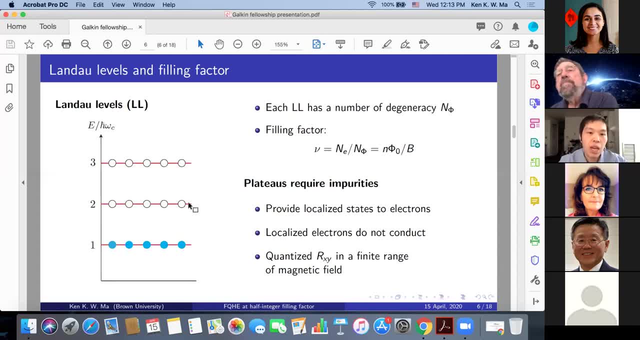 need a finite energy to excise the electron to a higher landau level and, as a result, the system is gap and we are in the integer quantum state. and since the energy is gap, then the bulk of the sample is insulating. now the energy is insulating and the bulk of the sample is insulating. now the 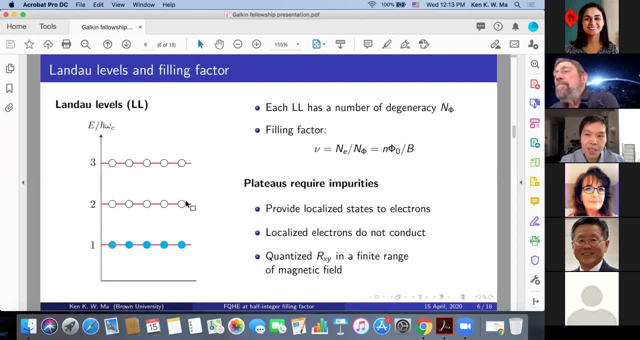 value of mu equals to the number of electrons that we can get. and when we do that, we get a finite energy. and as you can see, when i say finite energy in the dia hello you may ask me- i also noticed that there is a non-celo whole resistance, or a non-celo hall conductance, in fact. 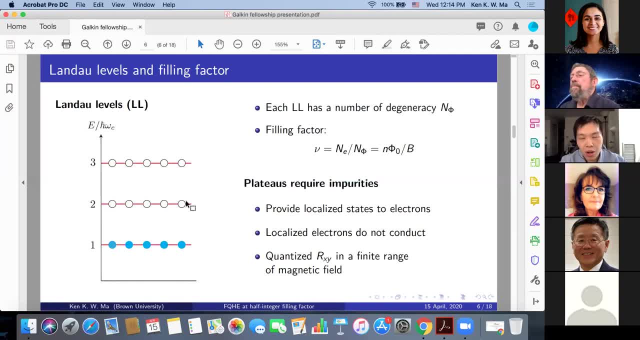 this comes from the edge of the sample and i will discuss it later. so the idea of landau levels may help us to explain the existence of a gap phase or individual quantum effect, but this does not. For example, we know that it is never perfectly clean. 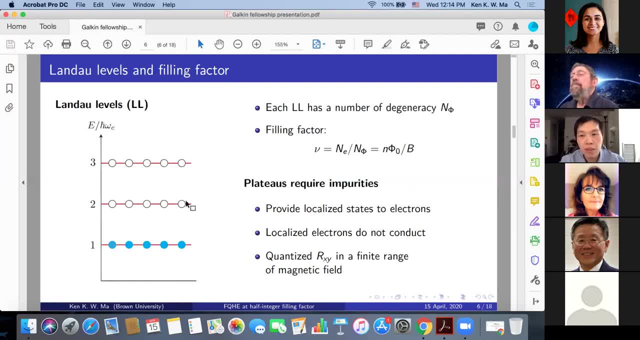 You must have impurity atoms or disorder effects, And these impurity atoms will provide localized states to electrons And electrons, during this localized state, cannot move freely, so they cannot conduct electricity And, as a result, they don't change the whole conductance. 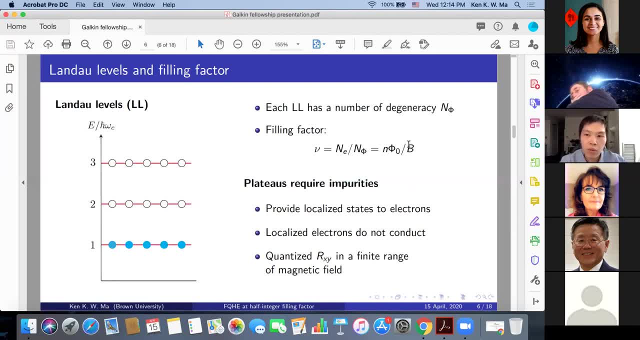 or whole resistance. Suppose I change the magnetic field a little bit, then this fueling factor changes a little bit and then the excess electron can go to this localized state and they don't change the whole conductance. That's why the whole resistance or the whole conductance. 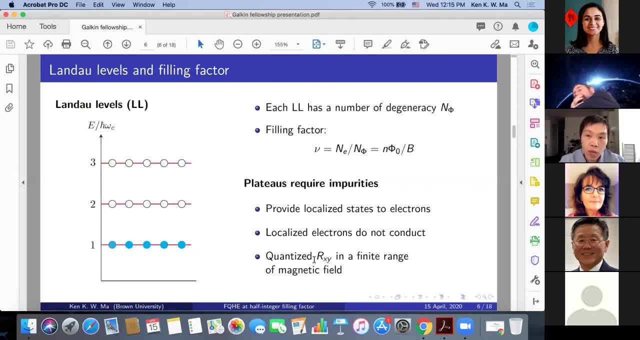 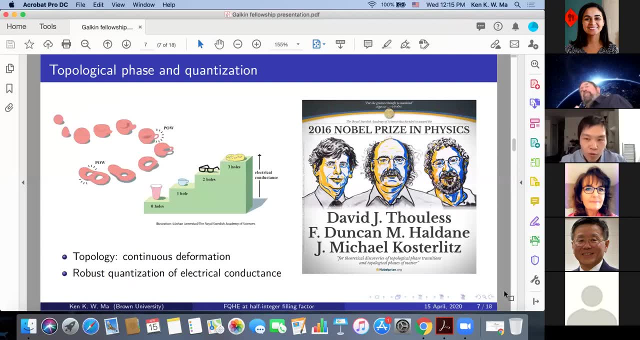 can remain at the same value over a final wave of magnetic field, and that's explain why they are exposed in whole resistance. Okay, in fact the whole resistance or the whole conductance are very precisely quantized and they are quite insensitive to the details of the materials. 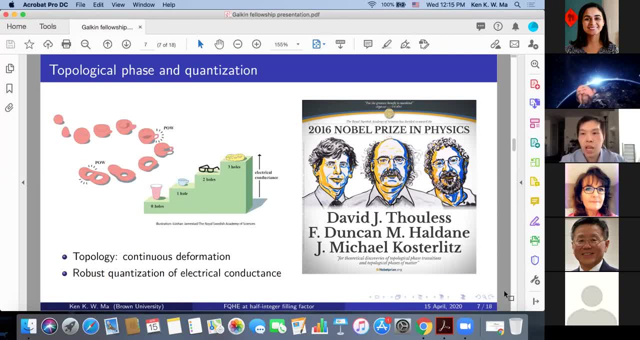 For example, it is insensitive to the shape of the sample, It is insensitive to the impurity atom profile in the sample. The underlying reason is that they are protected. I mean the whole conductance and the whole resistance are protected by topology. So in mathematics topology studies the global properties. 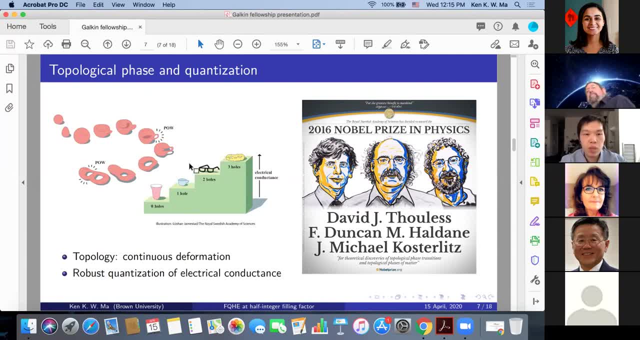 of a space. Two spaces are equivalent if we can deform one space to another space continuously. If we can deform one space to another space continuously. we can deform one space to another space continuously without making a hole there. Suppose I start from a ball. 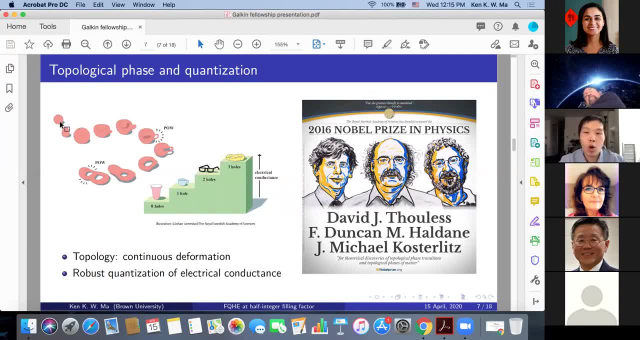 and then I stretch it a little bit to become an egg. then, according to topologies, these two shapes are equivalent. Now, if you don't agree with me and you feel very angry, you press the egg very violently and you generate a hole. 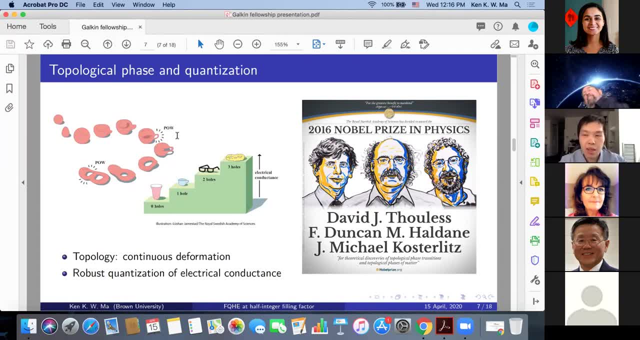 and change it to a mug with a handle, then at this time the topologists will also agree with you that an egg and a cup with a handle are topologically equivalent. Now in physics, we can also follow the idea of topology. 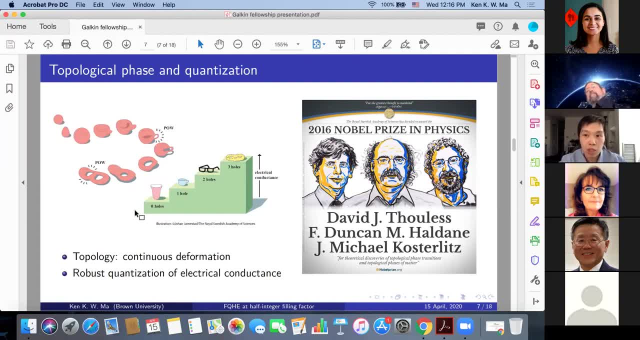 So if a physical quantity is protected by topology, it means that it is robust against more changes or perturbation in the physical system. As shown by Taurus and his collaborators, the whole conductance and the whole resistance are actually topological quantities. This explains why they are so robust against the small. 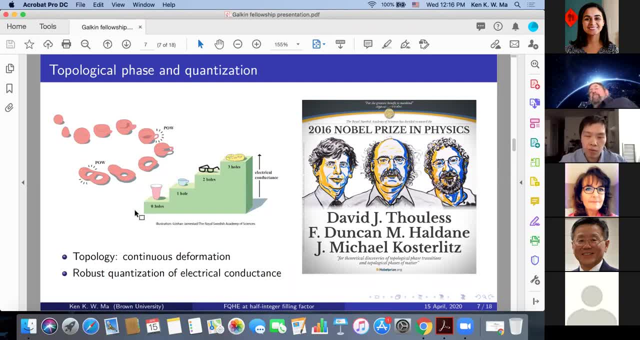 small details of the materials. I mean, they are so insensitive of those small details there. In fact, the Nobel Prize in Physics 2016 was awarded to Taurus Bourdain and Professor Korslis for their discovery of topological phase transition. 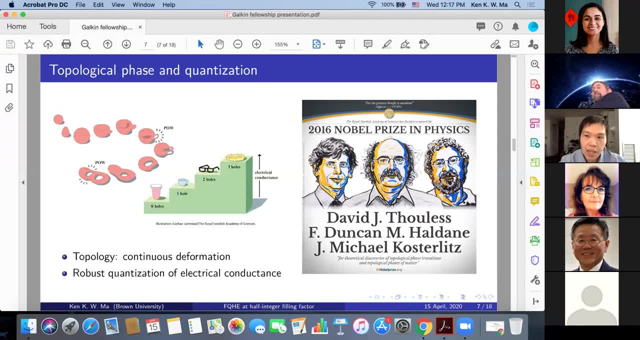 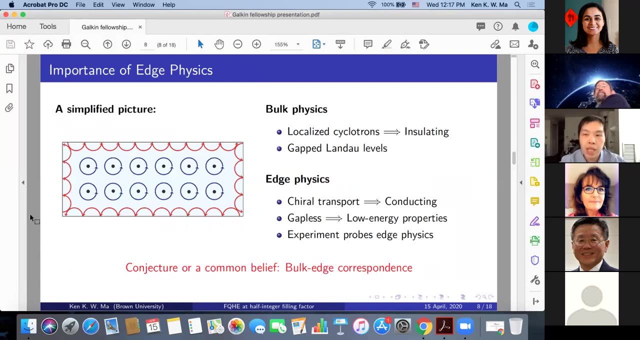 and topological phases of matter. As a student at Brown, I need to mention that Professor Korslis' office is just a few steps away my office- and I think he will agree with my comments here. OK, another important feature that I must discuss. 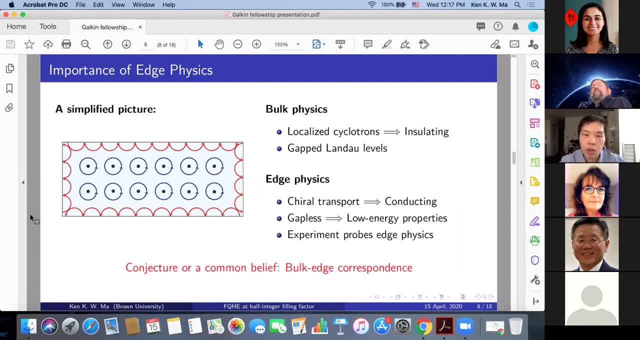 is the difference between the bulk and the edge of a quantum-hole liquid. This is important because I will discuss experimental probes to probe the nature of a quantum-hole liquid. Here I show you a simplified cartoon of the electron orbits in a quantum-hole liquid. 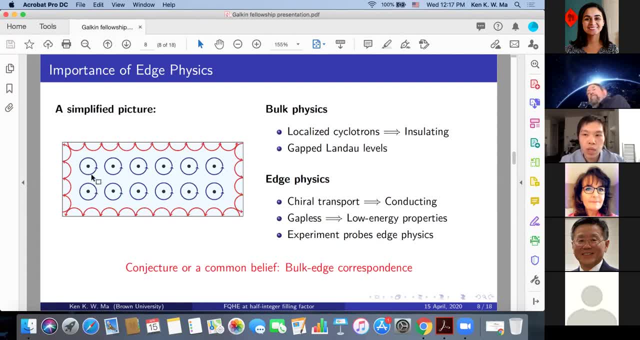 In the bulk, electrons are undergoing cyclotron orbits due to the magnetic field. As shown here, these cyclotron orbits are localized and electrons cannot move freely. As a result, the electrons in the bulk cannot conduct electricity and the bulk of the sample is insulating. 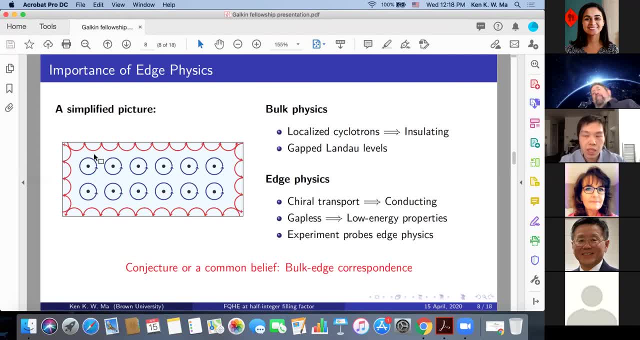 This conclusion agrees with my previous discussion based on Landau levels, But something different happens on the edge. Now the electrons cannot complete their cyclotron orbits. What they are doing is being reflected by the edge of the sample, So, as a result, they will continue. 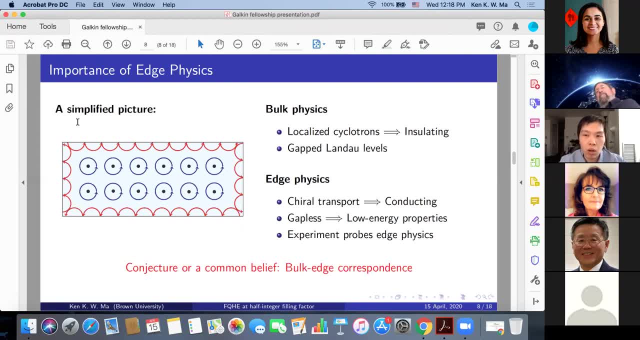 to move in a single direction. Due to the chirality or the single directional move of the electron, its best scattering, due to impurity on the edge, is strongly suppressed, So electric current can move along the edge of the sample And this explains why the whole conductance 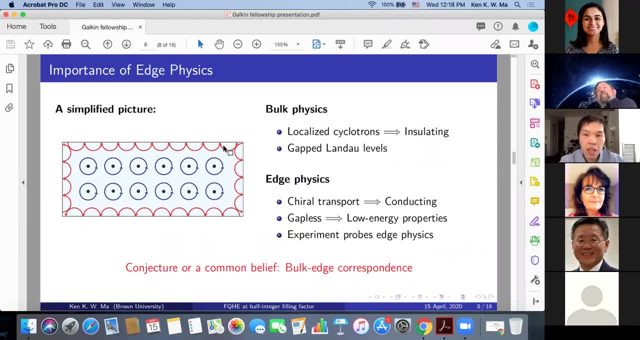 or the whole resistance is non-zero. Another important feature about the edge of a quantum-hole liquid is that it is gapless. In other words, it doesn't require any energy for us to excite an electron on the edge. In other words, it also means that the low-energy physics 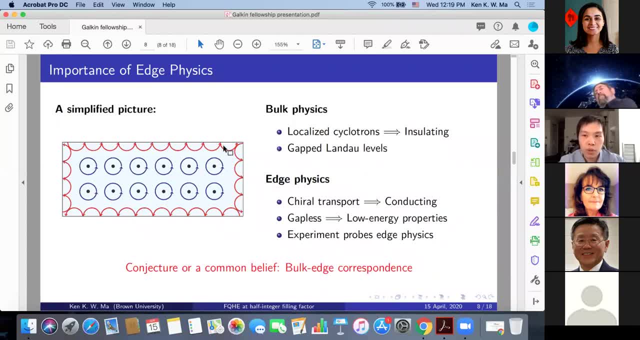 of a quantum-hole liquid is governed by the edge of the sample. So in an experiment we usually don't want to heat up the sample too much and destroy the quantum-hole state. So what we are probing in the experiment is the low-energy physics of the quantum-hole liquid. 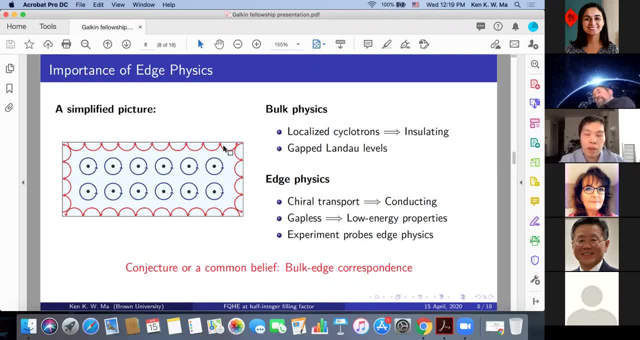 So we are probing the edge physics of a quantum-hole liquid. So at this moment you may challenge me: If I just probe the edge physics of a quantum-hole liquid, can I still learn about the bulk of a quantum-hole liquid? The answer seems to be yes, because we 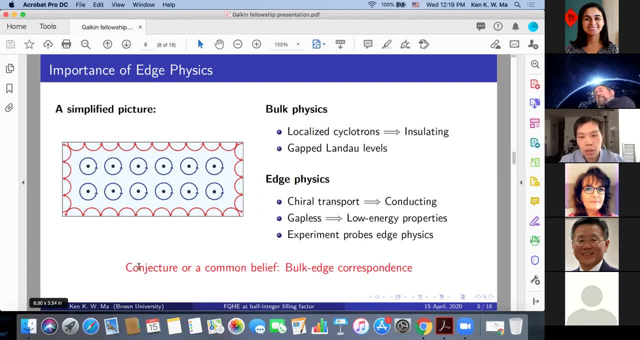 have a conjecture called the bulk-edge correspondence. This correspondence suggests that if we can understand the edge of the quantum-hole liquid, then we understand the bulk of the quantum-hole liquid automatically. So this is actually very good, because the bulk of the quantum-hole 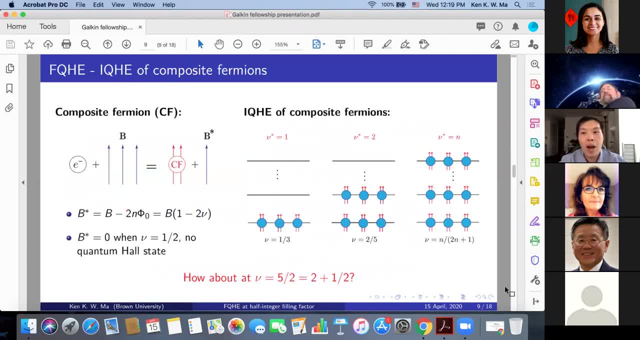 liquid is not in the same direction or in the opposite direction. So far I have just discussed why integer quantum-hole effects can exist and introduce some important features of integer quantum-hole effects. So how can we understand fractional quantum-hole effects In fractional quantum-hole effect? 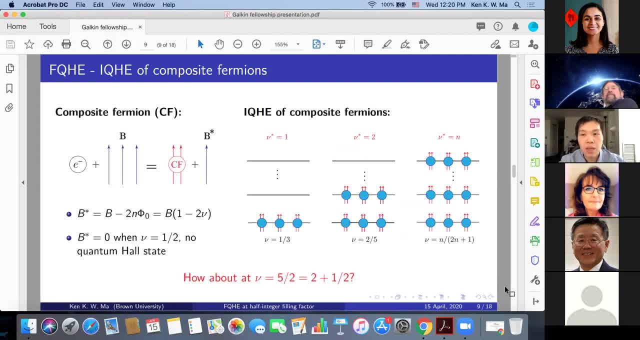 the fielding factor liu is now a fraction. the state should be gapless and we should not have any quantum Hall state there. However, the electrons in the sample are strongly interacting and the strong interaction of the electrons sometimes can open a gap in the Landau level and 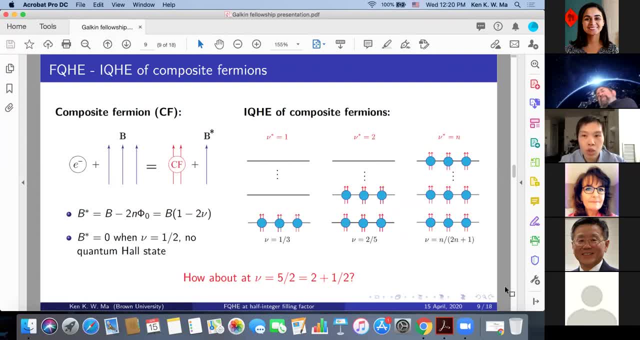 leads to a gap phase and leads to fractional quantum Hall effects. As I mentioned at the beginning of my talk, strongly interacting condensed matter system requires new approaches to understand it and describe it, and the theory of composite fermions is actually one of these approaches. In general, 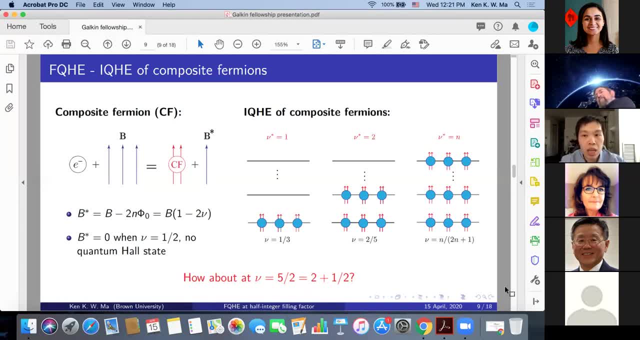 a composite fermion is formed by attaching an even number of magnetic flux quanta to every electron. Here I show you the example of attaching two magnetic flux quanta to an electron. Due to this, this force must meet the heat amounts, color, price event that are relevant to the harmonic vector values. 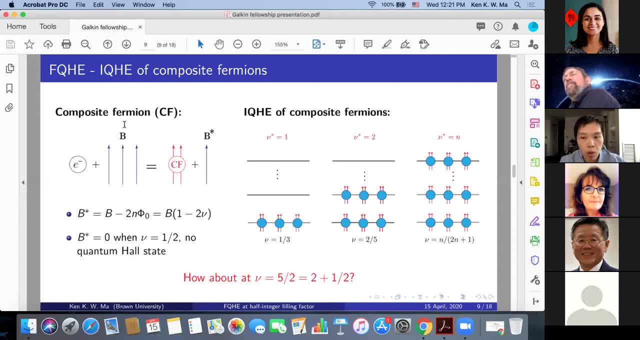 the effective magnetic field experienced by the composite fermions is smaller than the magnetic field experienced by the original electron. At the same time, the decrease of this magnetic field means that the effective fueling factor of the composite fermions is larger than the fueling factor of the original electrons. 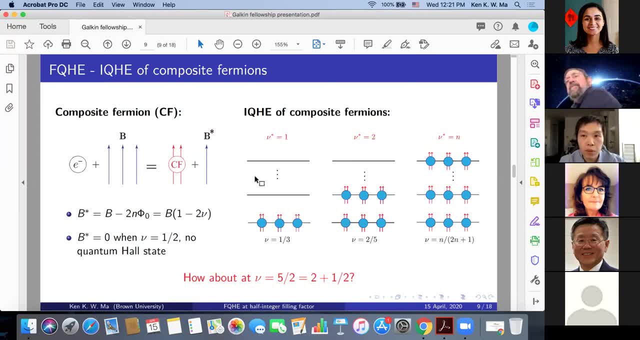 Suppose we have a completely filled and down level of composite fermions. If we do the mathematics correctly, this corresponds to the fueling factor: one third of electrons. Now I may repeat the same story If I have two completely filled and down levels. 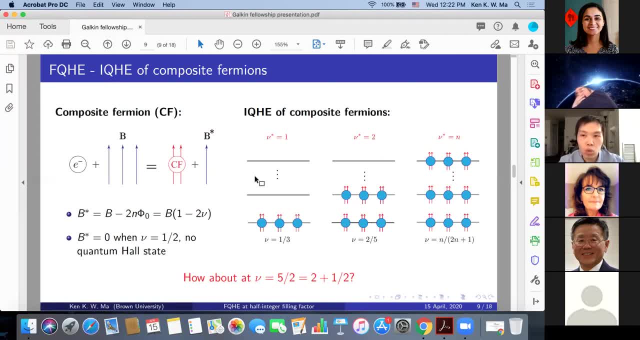 of composite fermions, it corresponds to a fueling factor two over five. If I continue to repeat this story, basically most of the fueling factors which have off the denominator can be understood in this way. Another feature for the composite fermion theory is that 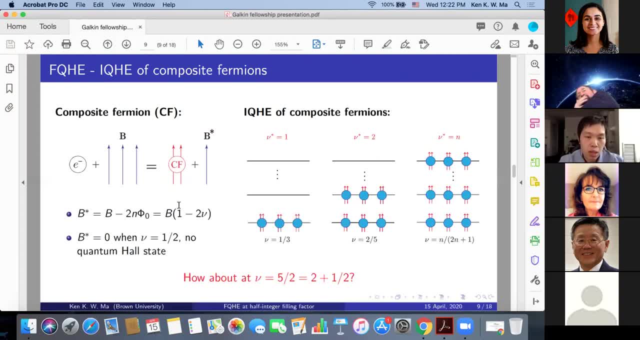 if we look back to the effective magnetic field, this effective magnetic field vanishes. I mean, this magnetic field becomes zero if the fueling factor equals to one over two. So in this case my system consists of a connection of composite fermions and there's no magnetic field. 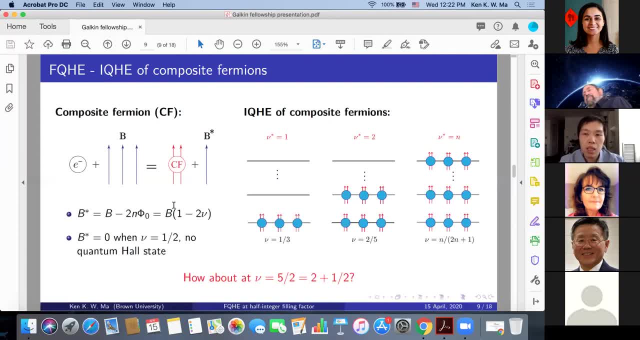 experienced by them. So, according to quantum mechanics, this composite fermion will just pile up in momentum space and then they will form a firm C. This system should be capless and there should be low quantum power. So this is the quantum state of the fueling factor one over two. 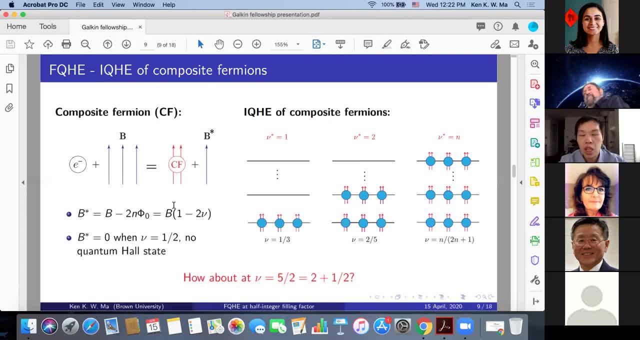 And this explains why there is no path close at nil equals to one over two or nil equals to three over two. A natural follow up question that you may ask is: how about in higher and lower level? Let's say what happens at a fueling factor of five over two. 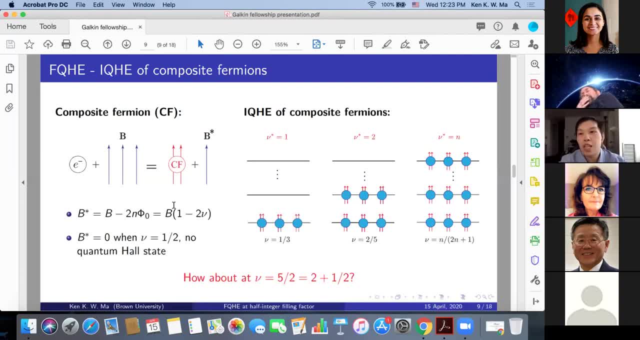 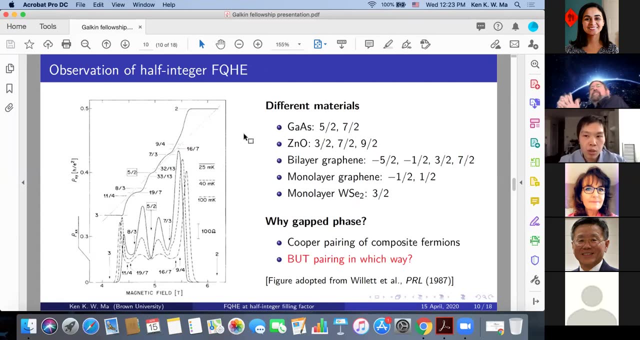 Naively. if we believe in the previous discussion, then there should be low quantum power state, the fueling factor five over two. But let's see what happens there according to the experiment. So physics always surprises us. On the left I show you an experimental data. 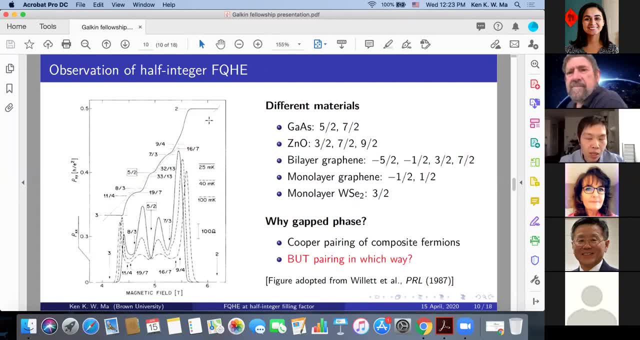 obtained about 30 years ago. As you see, in the Hall resistance we do see a very, very short path close in the Hall resistance. here, At the same position, we also see a minima in the longitudinal resistance. These two features tells us that there is actually. 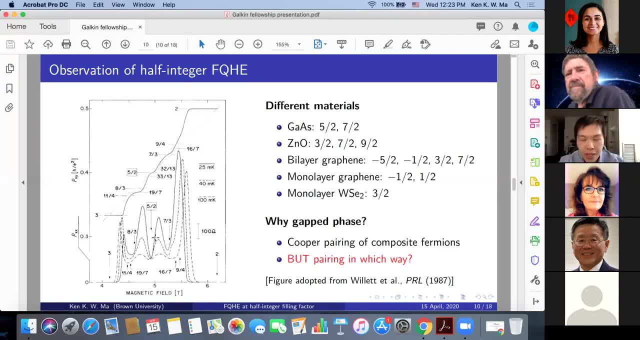 a fractional quantum state, In fact of five over two. Nowadays, 30 years have gone more half integer quantum Hall state can observe in different materials, including gallium, arsenide, zinc oxide, gold, monolayer graphene and bilayer graphene. 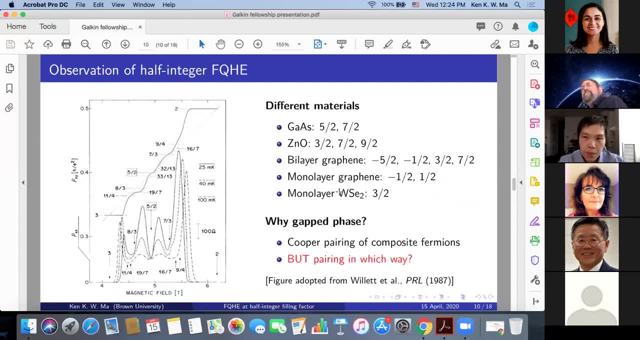 and most recently tungsten disalinide. So we do have some gap phase. We do have some fractional quantum Hall states at half integer fueling factor, But according to a composite fermion theory it cannot happen. So what's wrong here? 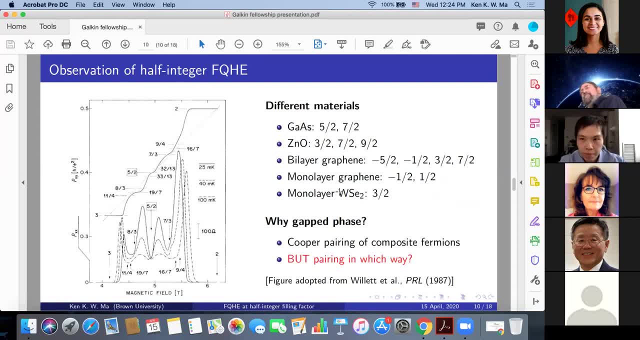 In fact we are missing an important ingredient. So for the composite fermion, sometimes they may also form proper pairs, just like electrons in a superconductor, And then, by forming proper pairs, it will open a gap in the system And this little gap phase. 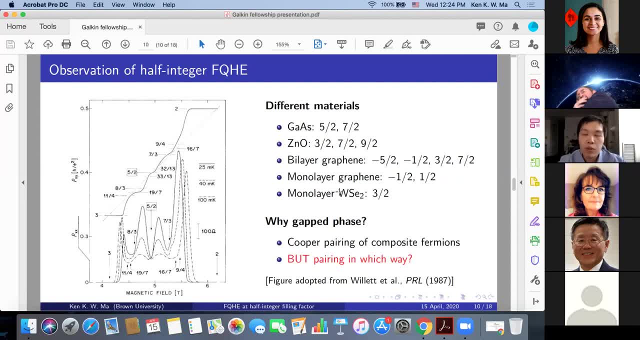 and this is exactly the origin of half integer quantum Hall. But now I didn't tell you how I should pair up the composite fermions. In fact, different ways of pairing the composite fermion will lead to different candidates, And this candidate we usually call it as topological order. 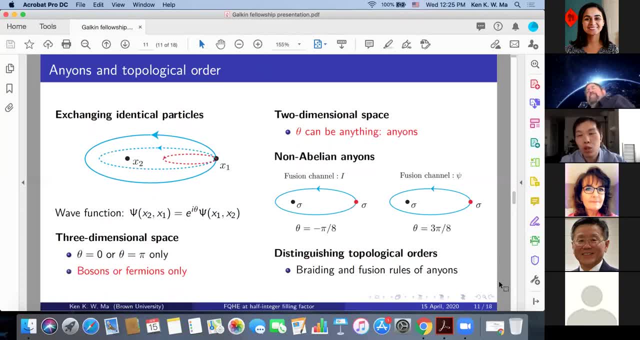 So, in order for me to discuss what is a topological order, I need to digress a little bit to introduce you to a concept called anion. So let's say I have a system called anion. So let's say I have a system called anion. 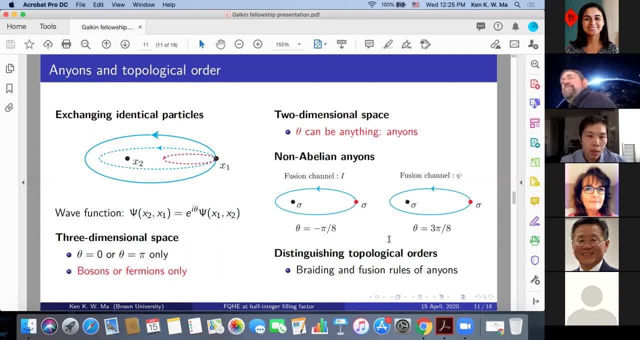 I have a system consisting of two identical particles. One of them is at position x1, another is at position x2. Now in quantum mechanics I can write down a wave function to describe this system. Suppose I want to exchange these two identical particles now. 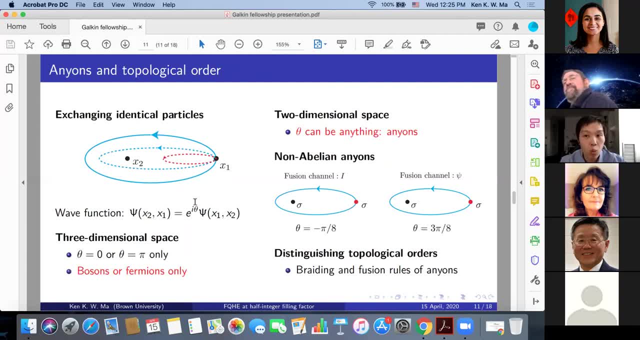 The result is that I will introduce a phase factor to the wave function. Now I want to study what are the possible values of this phase factor. In order to just look at exchanging a particle, let me look at another operation, that is, moving one of the particles around. 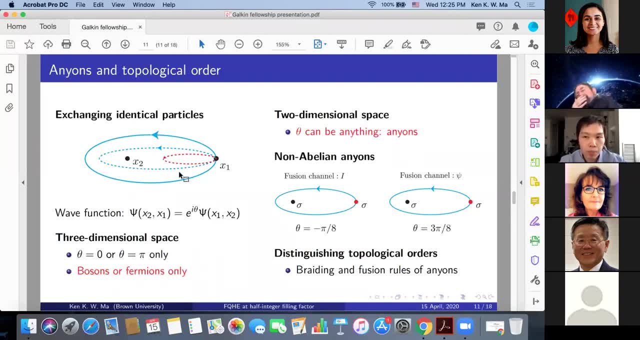 another one in a full circle. Now this operation is equivalent to exchanging the two identical particles twice. So I will obtain a value- two beta- for my phase factor. But this value is topological, meaning that I will still obtain the same value if I can deform the trajectory of the particle continuously. 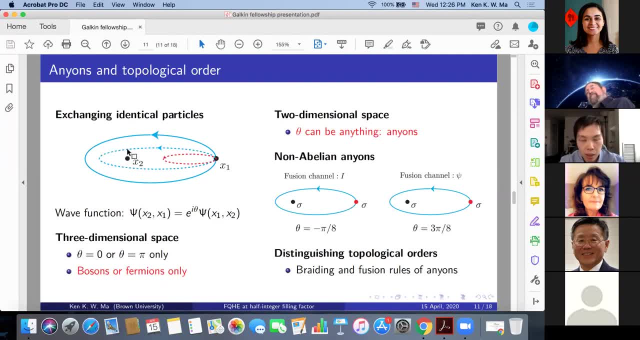 Now let us first focus on the phase in three dimensions. I can start from the full solid loop, as shown here, and then I can string it to a smaller loop, the full dash loop here, When this loop is very near to the second particle. 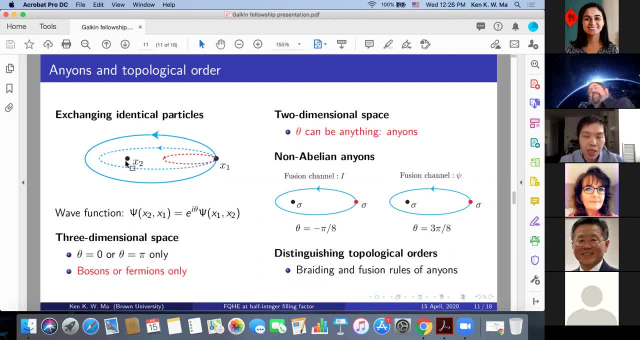 I can lift up the loop away from the two-dimensional plane, Then I can continue to string it to a smaller and smaller loop And eventually this loop before the second particle will be the same as before. So I can continue to string it to a smaller loop. 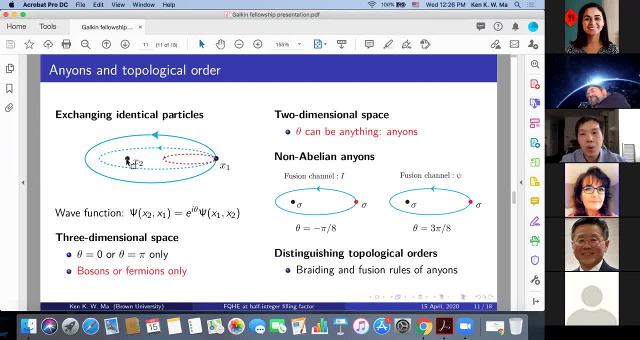 And eventually this loop before the second particle will be the same as before, And eventually this loop before the second particle will be the same as before, And then inside this point, basically we enclose zero particle there. So what we are doing is basically nothing. 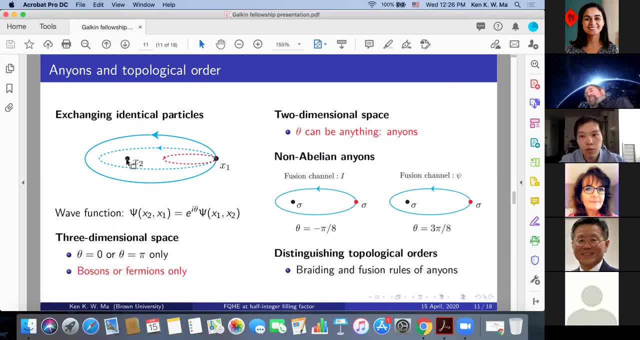 By doing nothing, we should get a phase factor. two beta equals to zero. So if we look back to exchanging identical particles, then we only have two values of beta, either zero or pi, because pi times two is two pi, but two pi is basically equal to zero. 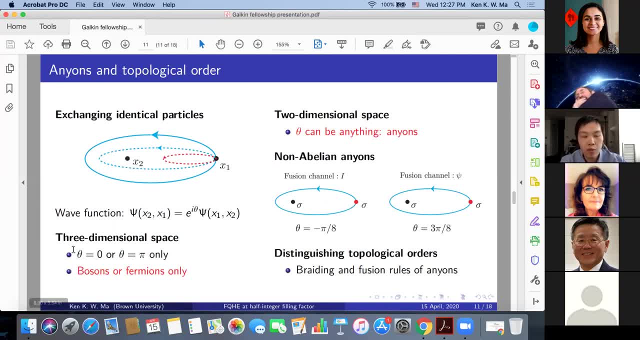 So in three dimensions I only have two possibilities: either theta equals zero or theta equals pi, and these correspond to bosons and fermions. Now, in two dimensions, my previous argument breaks down: At this time I cannot sink this blue solid loop. 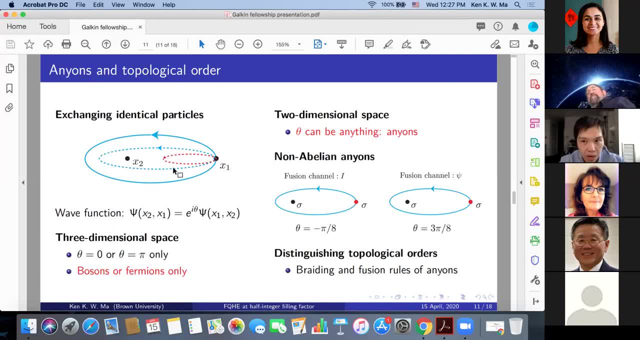 to this red dashed loop here without crossing a second particle. So theta- I mean the value of theta- can be any value in between zero and pi. That's why we call this particle as pi. That's why we call this particle as pi. 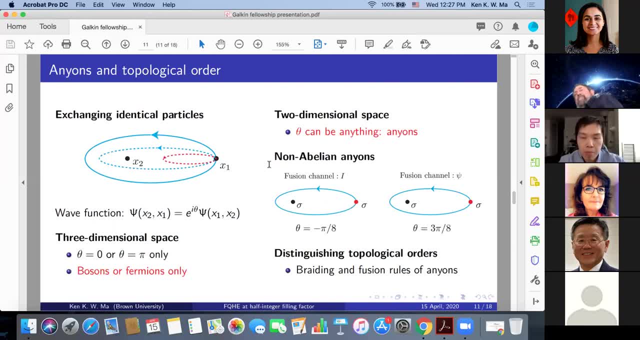 It. now. if I change these identical particles and you ask me what is the value of beta that you get, I can not tell you the answer until you tell me which configuration is returned to zero. my system want to be Loosely speaking. you may treat this configuration. 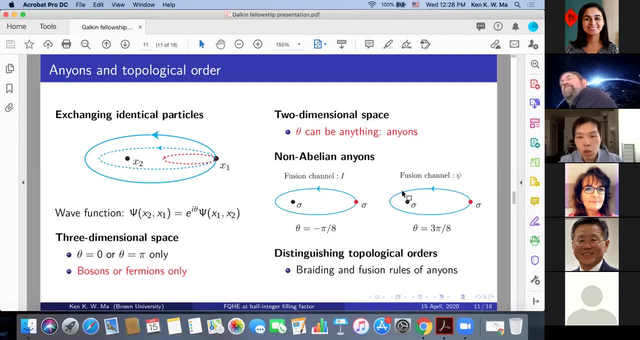 as an internal degree of freedom. Without telling you which configuration of my system want to be, I mean, without telling you which configuration these anions want to be, I cannot tell you what value of data I will get after exchanging these two particles. 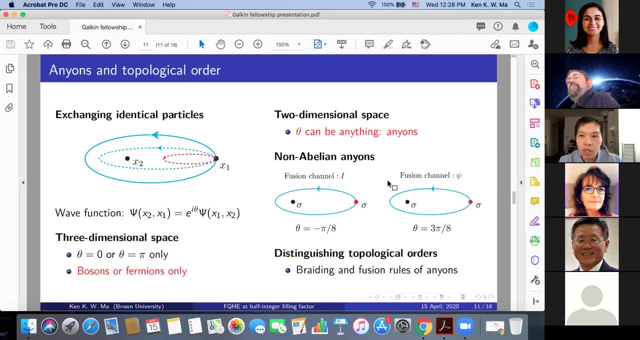 If this crazy situation happens, then we call these anions as non-abelian anions. Okay, so a topological order is defined by the value of beta that I will get by exchanging two identical anions and also what configurations that the anions can have in the system. 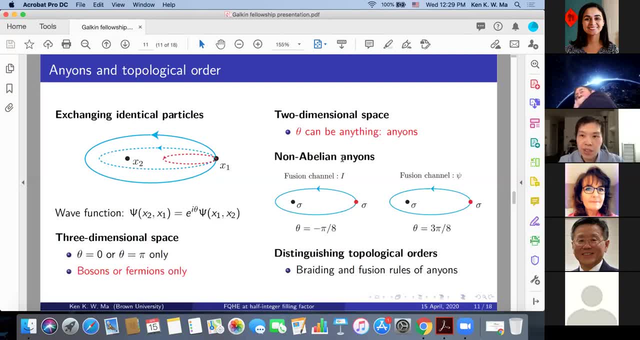 In other words, two topological orders or two candidates of fractional quantum host states are different if they have different values of beta after exchanging anions, or they have different configurations of the anions, If a topological order has non-abelian anions in the system. 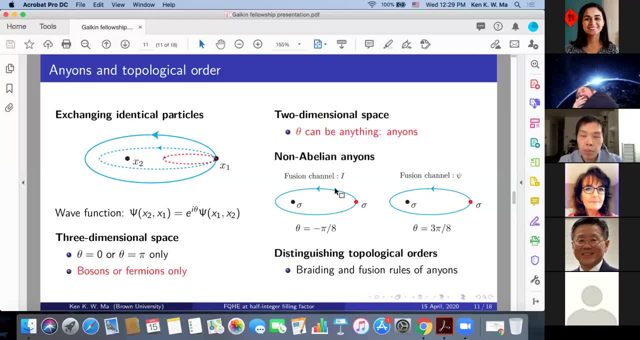 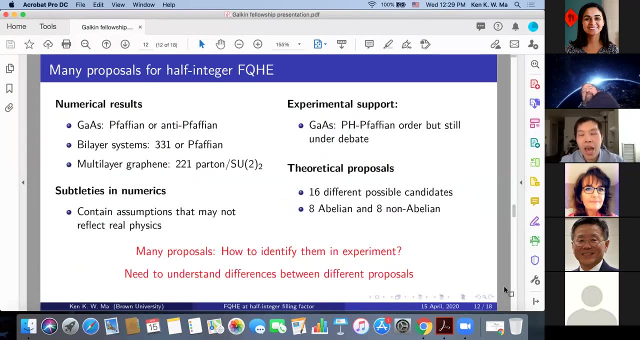 then we call this topological order as a non-abelian topological order. If the topological order doesn't have non-abelian anions, then we just call that topological order as abelian order. Now, after this definition, I can go back to the story. 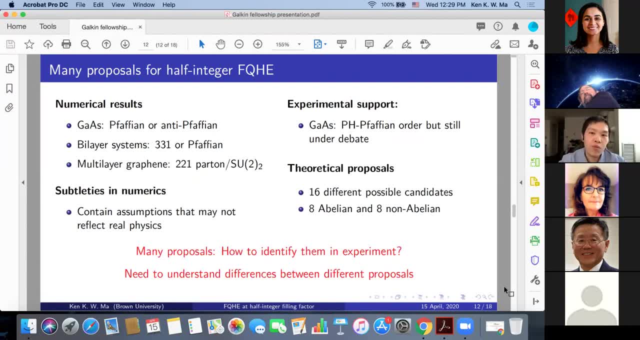 at fielding factor five, half in different materials. So in fact in a single-layer gallium arsenide, numerical results always support either the bargain order or anti-bargain order. However, another order called 3-1 is also suggested to be possible to exist in bilayer system. 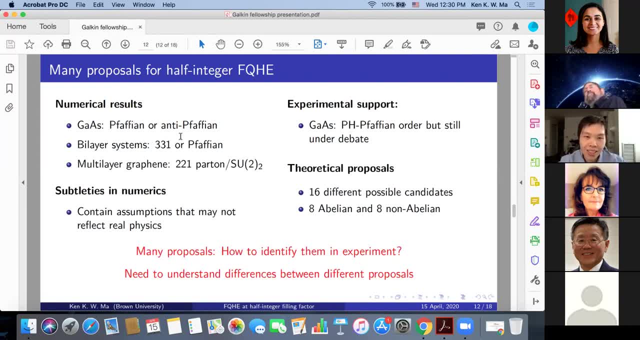 To make the problem even more supple, an other topological order: the 2-2-1 popcorn was suggested to appear in multi-layer graphene, So let me just focus on the single-layer gallium arsenide system Instead of the Favian or the anti-Favian order. 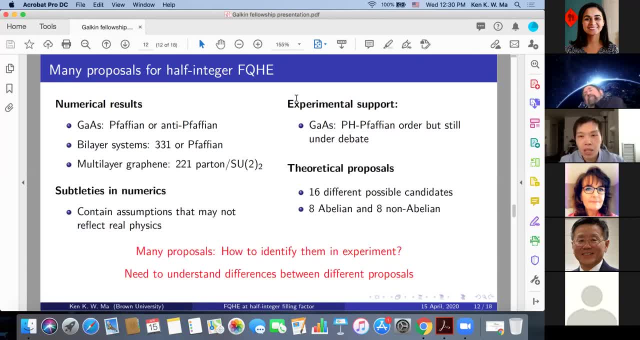 supported from numerical simulation. experimental data seems to support an other candidate, that is, the pH Favian order. So from here you see that there is a disagreement between numerical results and experimental data. So what happened here? In fact, in all numerical results, 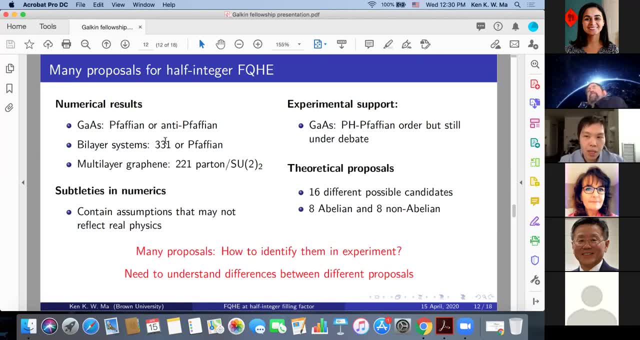 and in all numerical simulations we must need to make some assumptions, and these assumptions may not reflect real physics. For example, in a real sample I must have impurity, atoms and disorder effects, But it is very challenging for us to improve disorder effects. 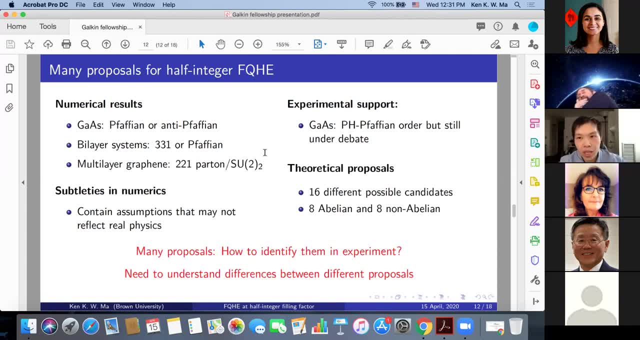 in numerical simulation If we just focus on theoretical ideas and theoretical proposals. Dima and I have shown that in particular, we can do it, But in fact we're not really doing it. So we can do it And I think who has the right solution? 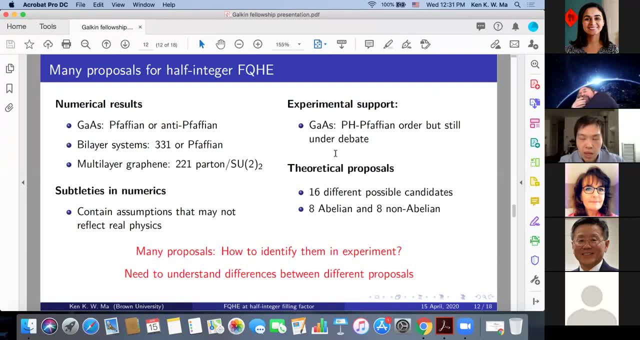 we can do it ourself, But in fact we can do it ourselves, For instance, for murder- neuen. there are many different algorithms that we can do. As I said, we have to be true to the principle that there are 16 different possible candidates. 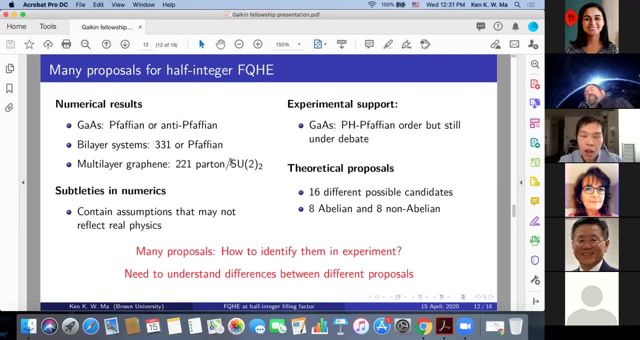 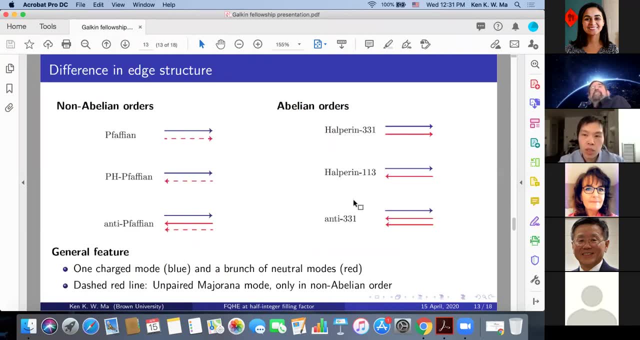 to describe fractional quantum power state as half-immigrant fusion factors. Each of them have nonlinear anions, but each of them not. Apart from the properties of anions in the system, different topological orders also have different edge structures. These agree with the bow-edge correspondent. 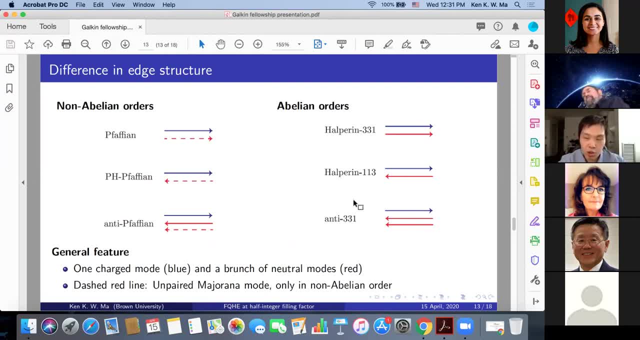 And the bow-edge correspondent tells us that if we load the edge physics then we load the bow. So if the topological order in the bow are different, then the edge physics should also be different. Here I show you some edge structure of some of the candidates proposed. 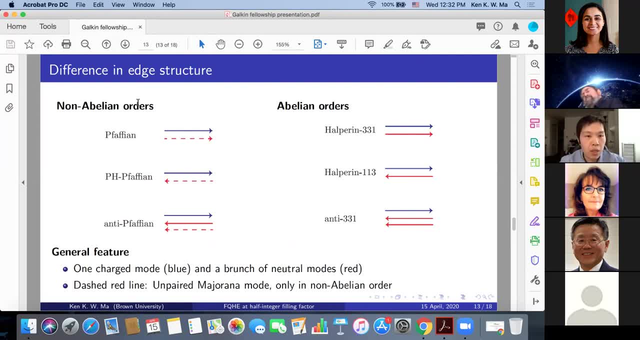 for the half-integer quantum host states. On the left, I show you three of the candidates which have run a billion anions. On the right, I show you three a billion orders. So, as shown here, all of them have a blue solid line. 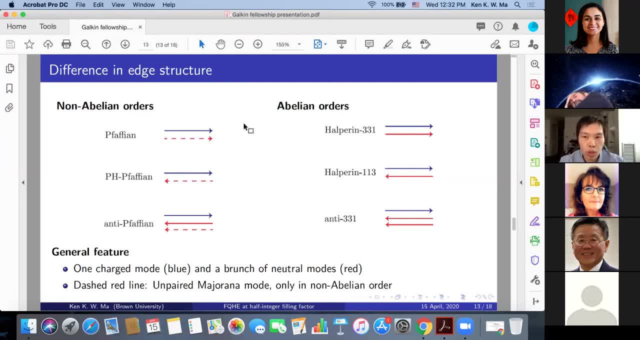 moving to the right. These correspond to the edge mode which carries charges And the main differences between the candidates here are the red lines. here They correspond to edge modes which are neutral, As shown here. this red line can move to the right. 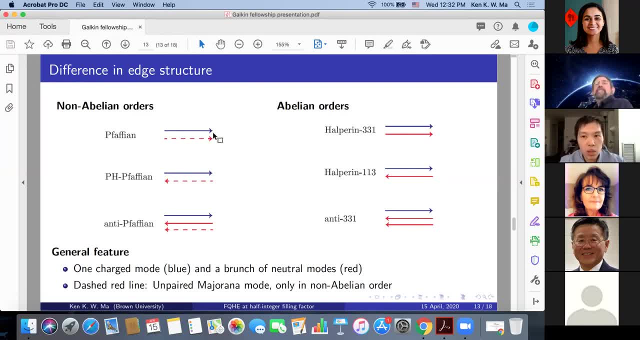 That is in the same direction as the charge mode. In this case we call this neutral mode as downstream. Also, this red line can move in the opposite direction as the blue solid line. In this case, we call the neutral mode as upstream. 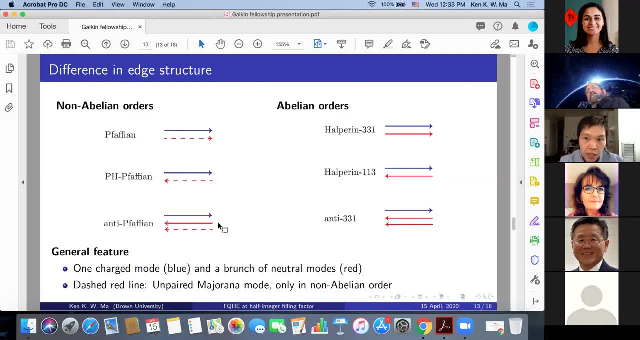 In addition, we also see that some red lines are solid lines, some red lines are dashed lines And red dashed lines only appear in run a billion orders. These red dashed lines correspond to unpaired Majorana edge mode And this only appears in run a billion order. 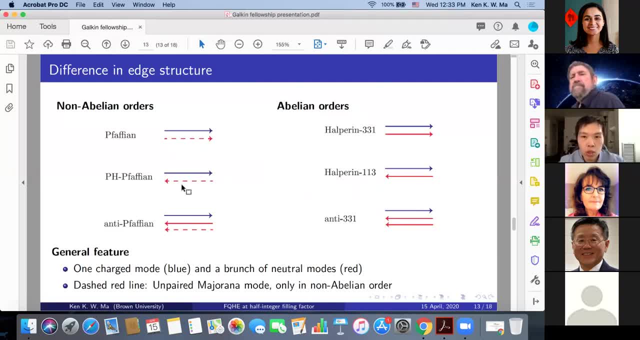 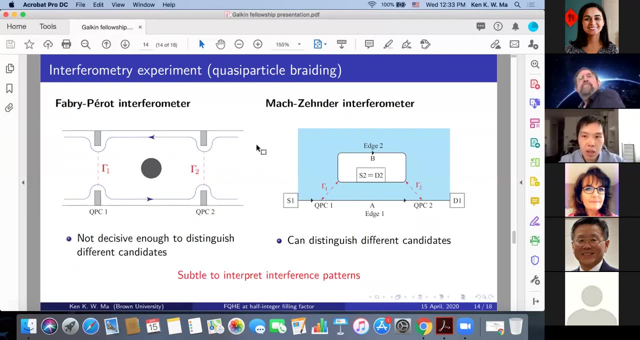 So if we can decide experiment which can distinguish different edge structure, then we may identify the relationship in different fractional quantum host states. So the first type of experiment make use of the differences in the anion properties in different topological orders. As I mentioned, different value of theta will be obtained. 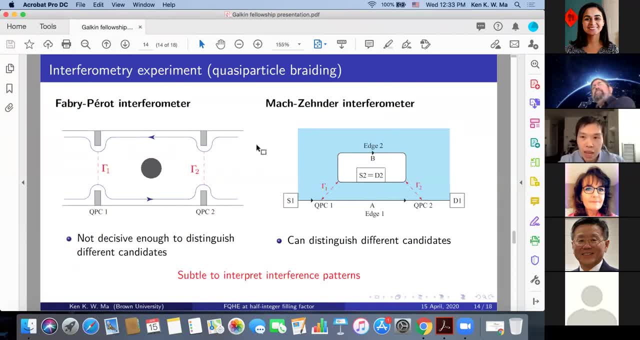 when I exchange different, when I exchange identical anions in different topological orders. So the first lateral type of experiment comes from interferometer. So in this type of experiment we make some level of regions such that the particles can tunnel from one edge to the opposite edge, as shown here. 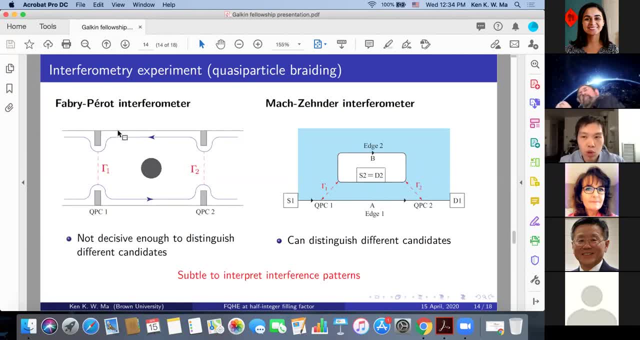 Now, if we make two such level of regions or quantum point contacts, then these particles can tunnel either at quantum point contact one or quantum point contact two. This leads to two different particle trajectories and lead to interference effects. What we are measuring in the experiment? 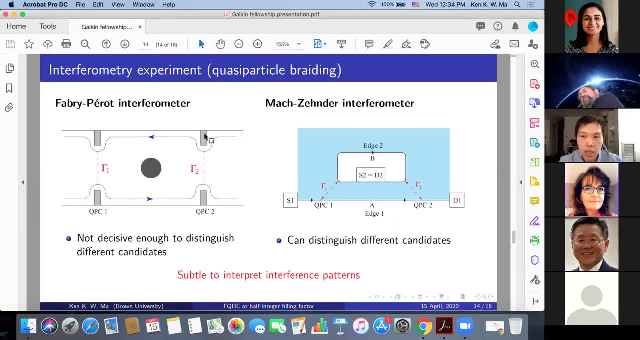 is the electric current due to the tunneling of particles in the interferometer. So the first type of interferometer we have is the Fabry-Perot interferometer. At the beginning it was suggested that this type of experiment may help us to distinguish between non-abelian orders. 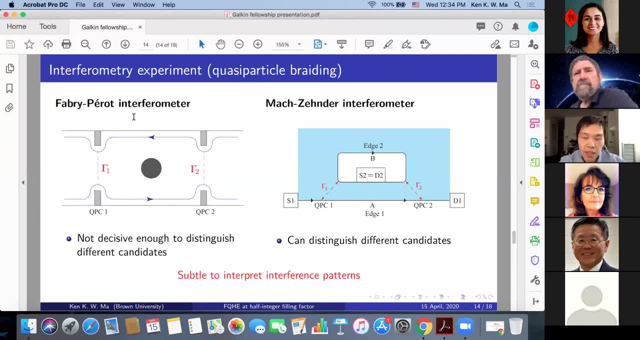 and abelian orders. But later work showed that it does not in some circumstances. So in other words, Fabry-Perot interferometer may be not decisive enough to distinguish different candidates for fractional quantum state at half integer fielding factors, So we need an other type of interferometer. 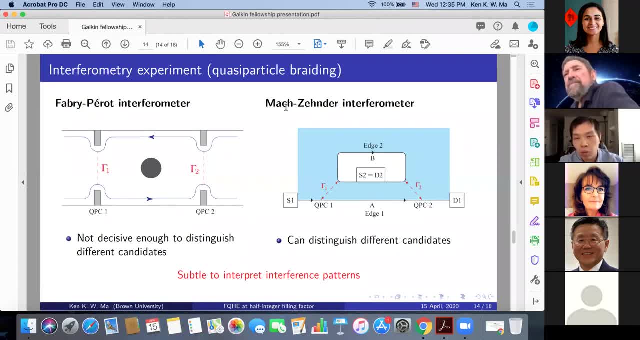 Here. another type of interferometer is the Maxander interferometer, Similar to the Fabry-Perot interferometer. particles can tunnel between opposite edges at these two quantum point contacts, or these two level of regions, and set up an electric current, Hema, and I assumed that for all 16 topological orders. 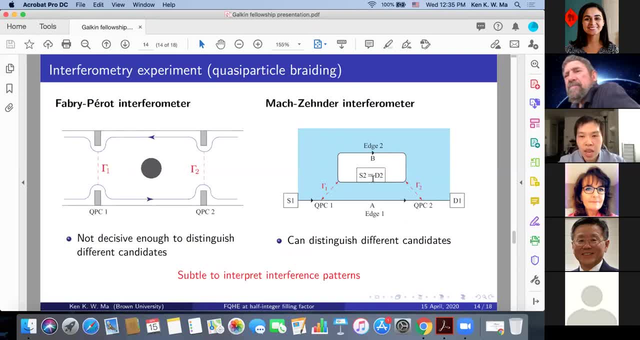 they will show different tunneling currents in a Maxander interferometer. Also, the noise in the tunneling current are different for each topological order, meaning that you will get 16 different tunneling currents as 16 different noises in the current for those 16 candidates. 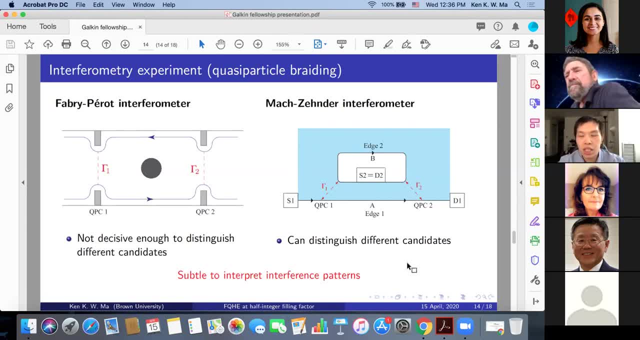 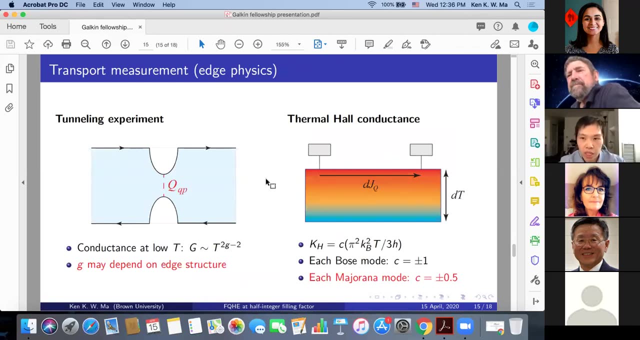 However, at this moment this is still very challenging and supple to analyze the interference patterns or the experimental data from interferometry experiment. At this moment, more useful information comes from transport measurement. In this kind of experimental technique, what we are hoping is the edge physics. 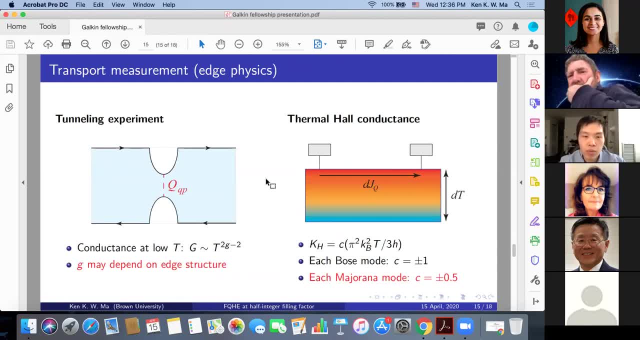 of the quantum power electric. The first type of experiment that we may do is something called tunneling experiment. Similar to previous type of experiment, particles can tunnel between opposite edges in the level of region and set up a tunneling current. So what we measure in the tunneling experiment, 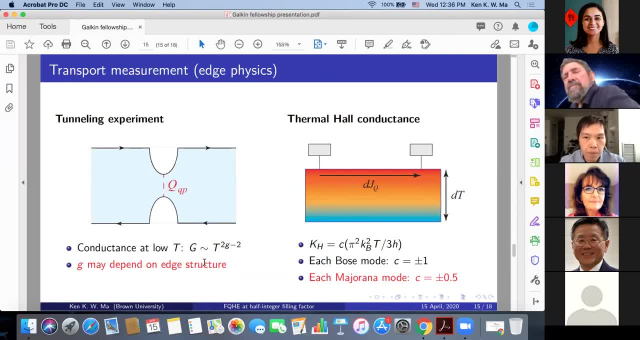 is the electrical conductance big G, as shown here, At low temperature. this big G is predicted to scale with temperature in this form and we want to measure the small g here. This small g will depend on the charge of the particles. 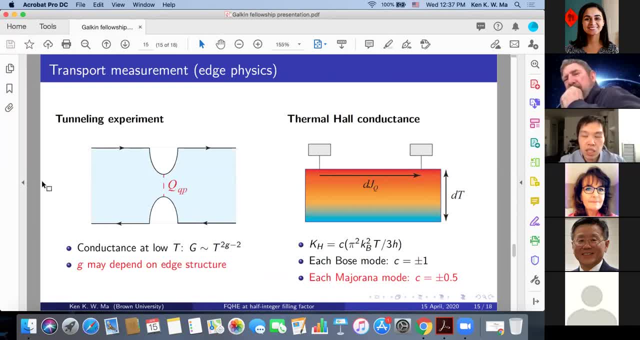 which participate in the tunneling event. In some cases this small g will also depends on the edge structure. If this happens, then by measuring G we may learn about the edge structure of the quantum power, electric. then we may learn something about the nature. 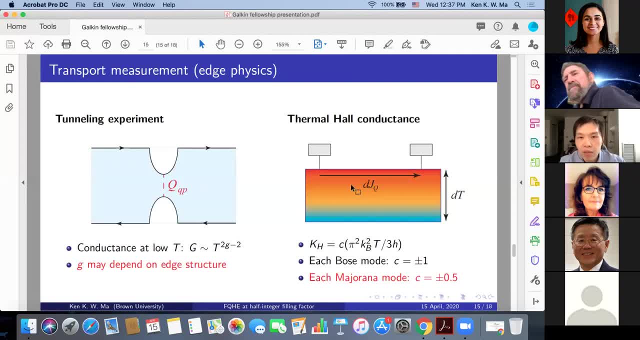 of the fractional compost state And other type of transport measurement that we can do is thermal conductance experiment. Suppose I apply a temperature gradient to my sample, then it will flow along the edges and the thermal conductance will depend on the edge structure. 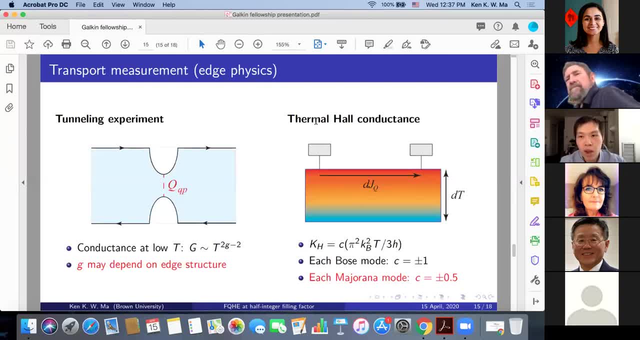 of the quantum power liquid and set up a thermal current. So the thermal conductance is defined as the ratio between the heat flow and the temperature gradient that applied to the sample. And this thermal conductance is predicted to take this form and there is a very important constant C here. 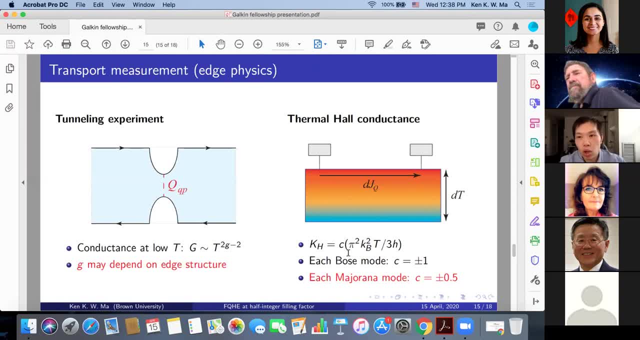 This C will depend on the edge structure of a topological liquid. If the topological orders just have solid light- I mean just the picture I shown you previous, slide later- if the edge mode is really centered by solid light, that is a both mode- then the value of C. 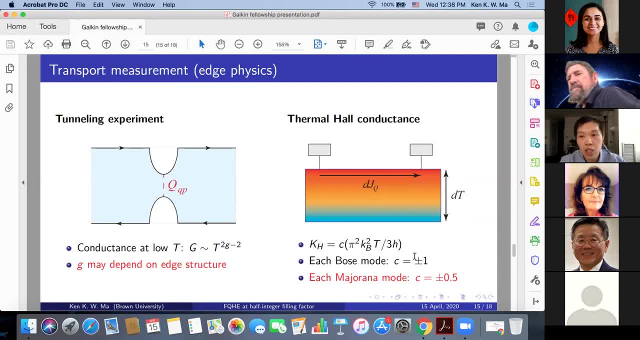 can only be plus or minus one The side depends on what direction this mode is traveling. And more important feature is that if I have a red dashed line, that is, if I have an unpaired minor runner mode which only appear in Ronnebian order, 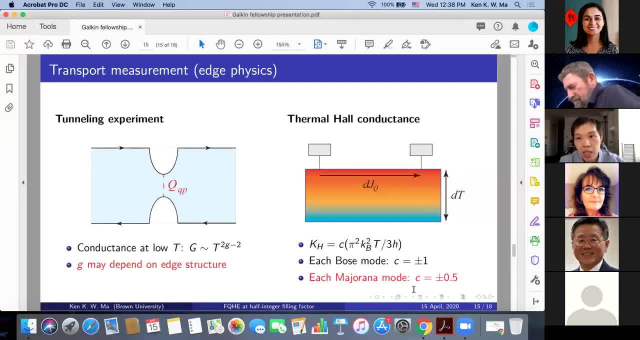 then the value of C can only be plus or minus 0.5.. Now, in general case, in a general case, I will have more than one edge mode on the quantum power liquid, and then I need to add up these different contribution. 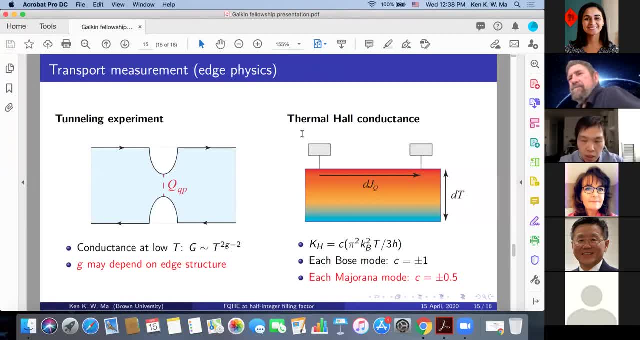 to obtain the value of C in the thermal power conductance. But no matter how you do the addition or subtraction, if you just do an addition or subtraction of integers, then you will still get integer. And but I show you that in Ronnebian order. 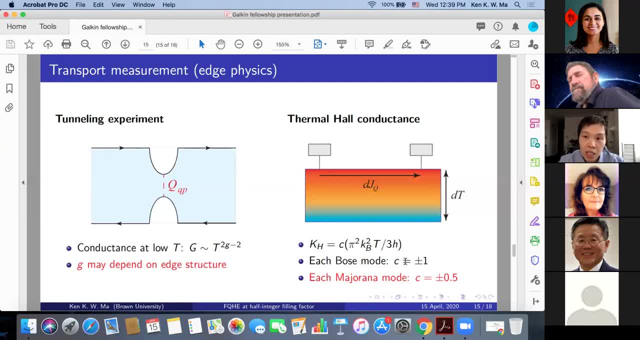 I only have one red dashed line: By adding integer to a half integer, I must get a half integer. So if you measure a half integer thermal power conductance, this is a strong signal that your system has a Ronnebian order. So in principle you may say: oh well, okay, okay, okay. 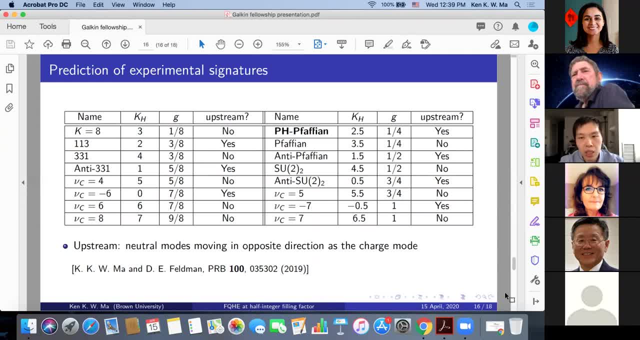 So you may summarize different experimental signatures predictor for all 16 topological orders in different experiments. Yima and I have done that And here I show you the table. Here I just show you the thermal power conductances predictor for each candidate. 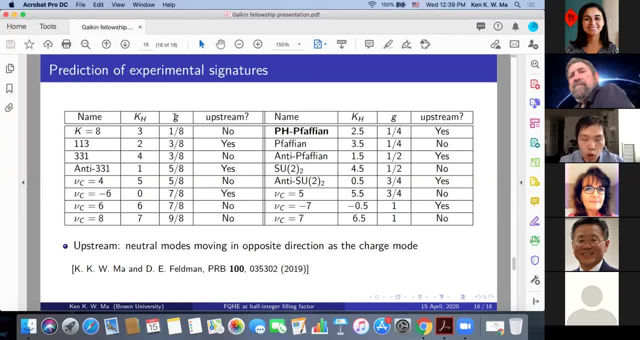 and also the small value- I mean the value of small g for each candidate, and also whether those red lines move in the same direction or in the opposite direction as the charge mode. That means the blue solid line. So using this table in principle, 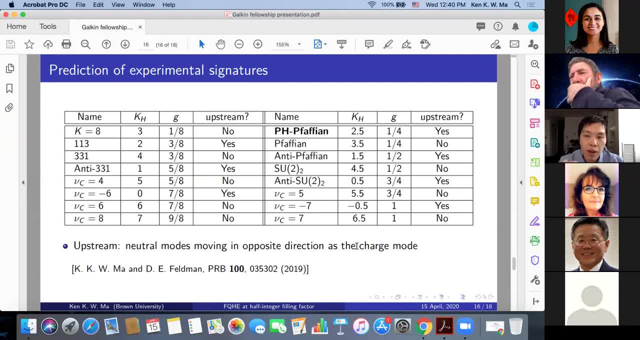 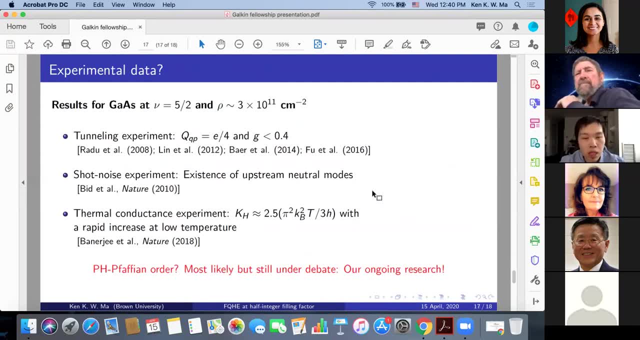 we may identify different candidates for the five half states in different materials. So let's see what experiment tells us. Here I show you some experimental data obtained for gallium aconite at the fueling factor five half at this electron density. If you go back to my previous table, 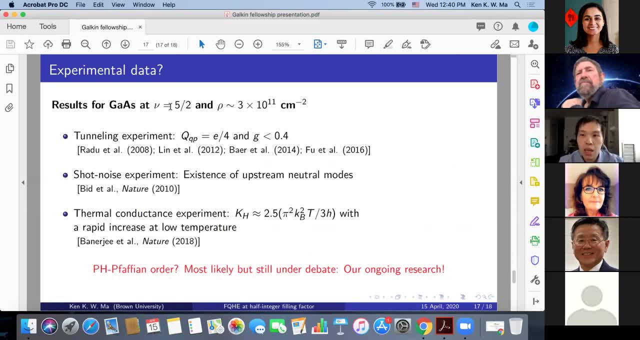 then only the pH five in order can agree with all these experimental data in a natural way. Even more special is that the tunneling experiment actually eliminates anti-Farbian order And the existence of upstream neutral modes eliminated the Farbian order. So you see both Farbian and non. 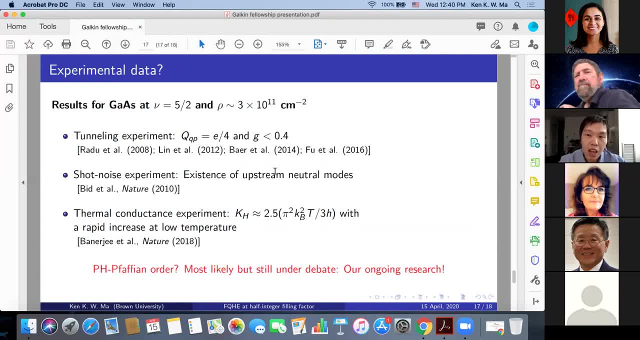 I mean both Farbian and anti-Farbian order have been eliminated, and these two candidates are supported by numerical simulation. So it seems that the most likely topological order to describe the five half states in gallium aconite is the pH Farbian order. 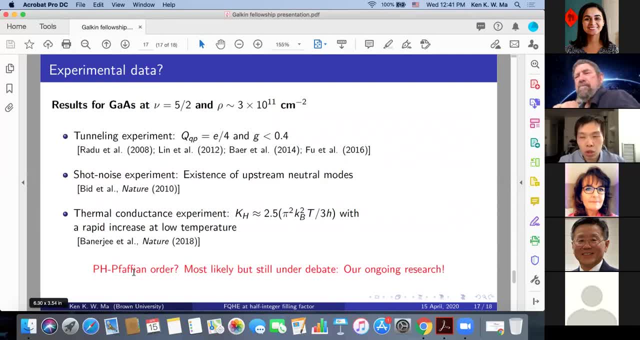 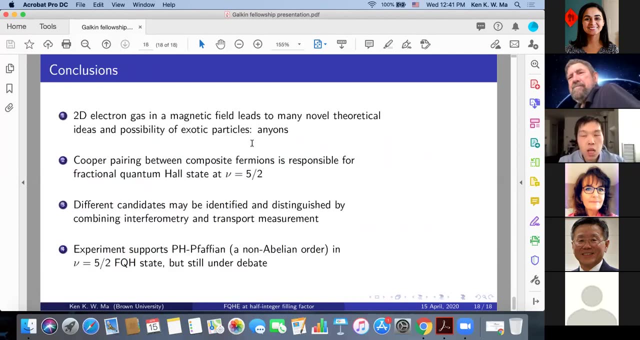 But there is still on the debate. There are alternative interpretations of the experimental results, And this is exactly our ongoing research: to see which interpretation is the most natural and the most convincing. So, to conclude, I would like to conclude that fractional quantum Hall effect may appear. 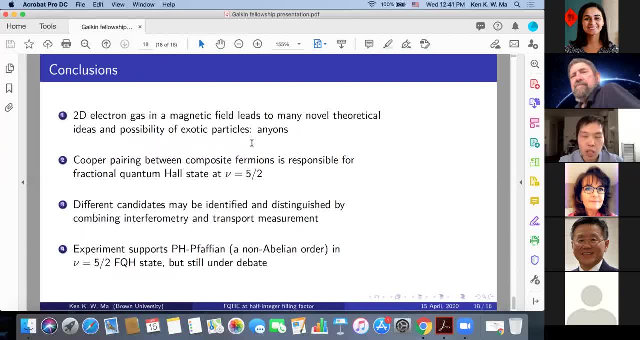 if I have a two dimensional electron gas and then place it in a strong magnetic field and pull the system to a low temperature. And the discovery of fractional quantum Hall effect leads to many low-flow theoretical ideas, such as the possibility of having andeons. 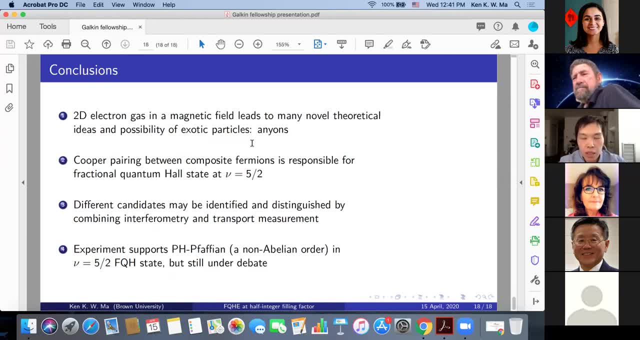 I mean the possibility of realizing andeons And then the five half states or other half integer quantum Hall states are so special because they require copper pairing between composite thermoids. Here different ways of pairing the composite thermoids will lead to different possible candidates. 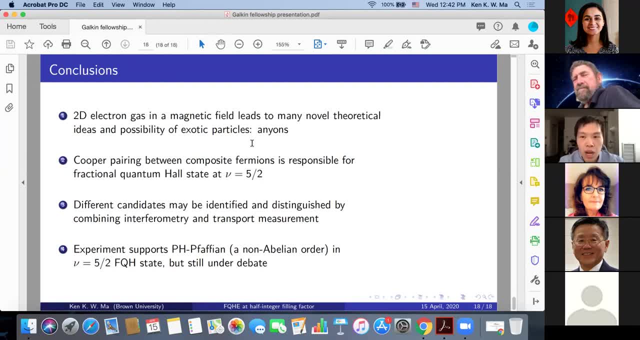 for half integer fractional quantum Hall states and the nature of the half integer quantum Hall states can only be revealed from experiments, And we can do interferometry experiment and transport measurement. By combining these experimental results we may identify the nature in different half integer quantum Hall states. 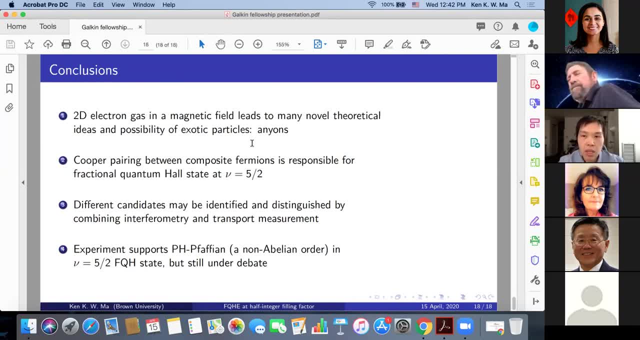 and by combining these experimental results, different half-individual compost states, especially the five-half state in gallium arsenide. And then, at this moment, the existing experimental data seems to suggest that the pH-5 gain order is the most promising candidate for the five-half state in gallium arsenide, but its nature is still 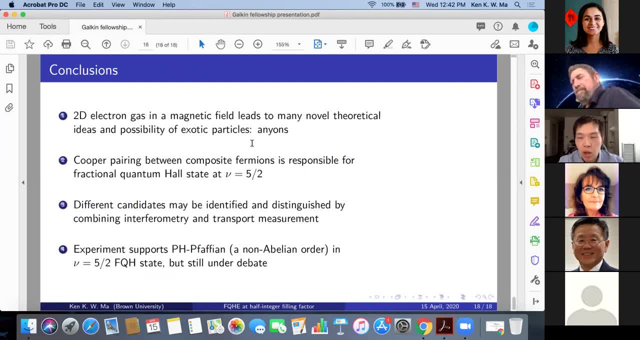 under debate. There are alternative interpretations and we need more researches to pin down which chronological order and which candidate is the most promising, the most natural and the most convincing. That's the end of my talk. Thank you Fantastic. Thanks a lot. Thanks, Ken. 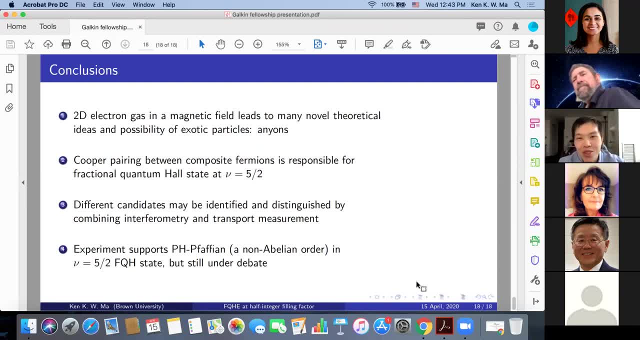 Okay, so do we have something like an A-section? I wonder if there are any questions. So I guess everyone is muted, right? Everyone's muted. Yep, maybe they could use the chat button. I think people can raise. people can raise their hand. Yeah, raise hand. 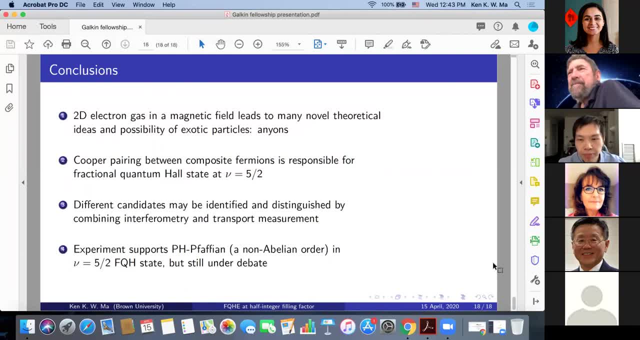 Raise hand or use the chat for a question if anyone has a specific question for okay, Hi Darshal, Hello, Hi, Hi. So you have a question. I think Professor is trying to ask a question, but he's muted. 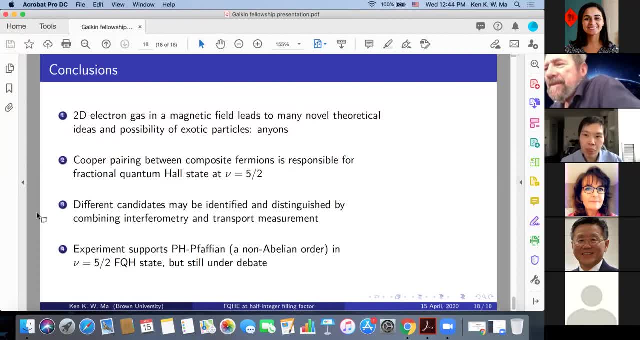 Let's unmute him. There we go. Go ahead, Mike. Hi there. So I'm muted, am I Okay? You are, you're unmuted now. If you have a question, go ahead. Okay. thanks When you say the experiment supports this particular pH-Prafian state. 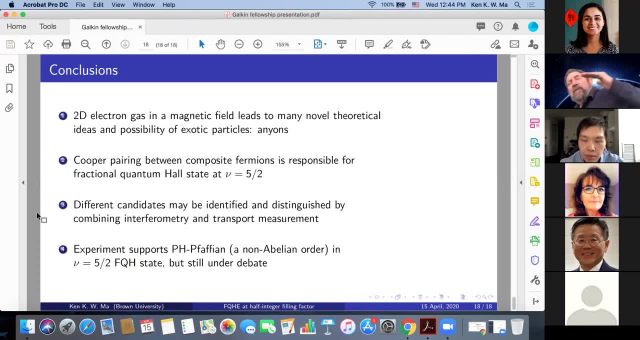 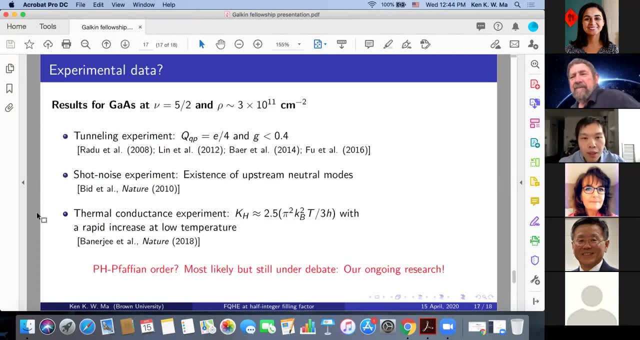 what you know. what exactly does that mean? I mean, what's measured, I see. So let me show you back what we get for the experimental data. The first experimental data we get is the small g should have a value smaller than 0.4.. 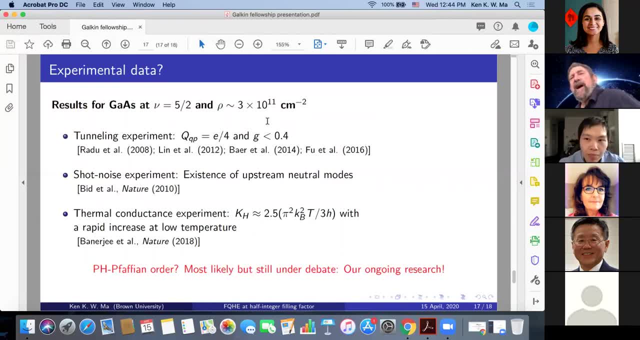 How accurate is the experiment? I thought that the various states required a knowledge of what you know. if you want to verify by experiment, you need to know what g actually. you know the value of g itself If you want to really know what state it is. 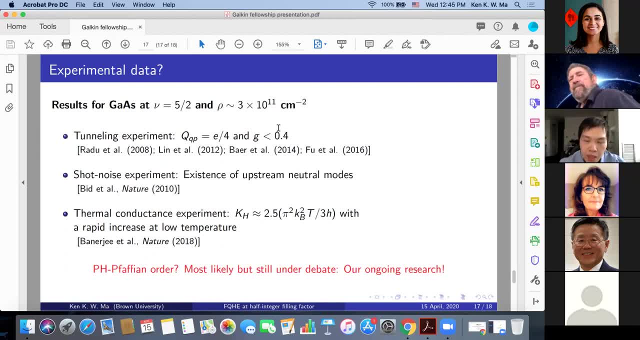 Well, you can only get an upper bound for g. unfortunately the reason is Coulomb interaction on the edge. Field theory always ignores it because it tries down short range local theories, but real life cares nothing about it. It's not a very long range and at 1000 you can get only an. 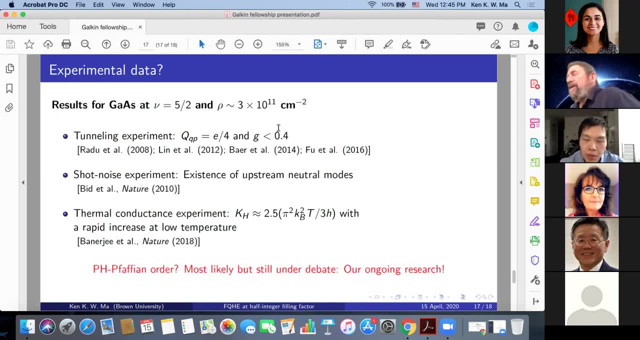 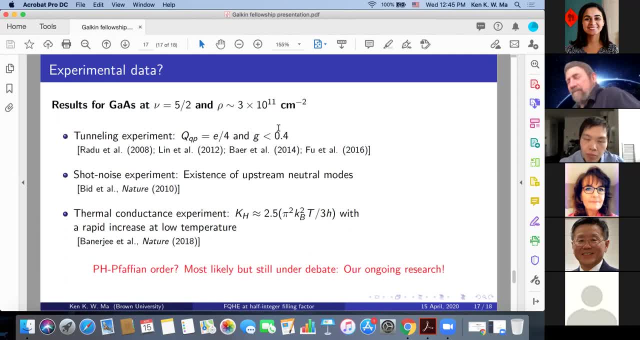 Yeah, Yeah, Yeah, It's in the universal number. You change gate voltage, g flows, So theory not good enough. It's not what Shaogang Wen was selling us 30 years ago. This g is the very first idea: how you identify topological orders. 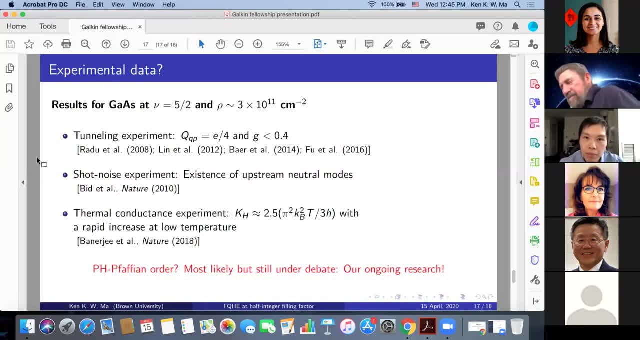 But if you write a nice local field theory, it tells you everything. The problem is that there is no single sample in the world that's discussed with this nice local field. The problem is that there is no single sample in the world that's discussed with this nice local field. 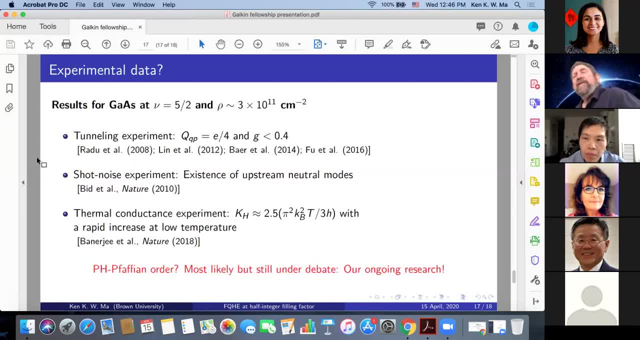 The problem is that there is no single sample in the world that's discussed with this nice local field. It's the same thing as after the K? It's the same thing as after the K. Okay, actually- and I was just asking the question- you can use a little theoretical theory of the state of the opponent. 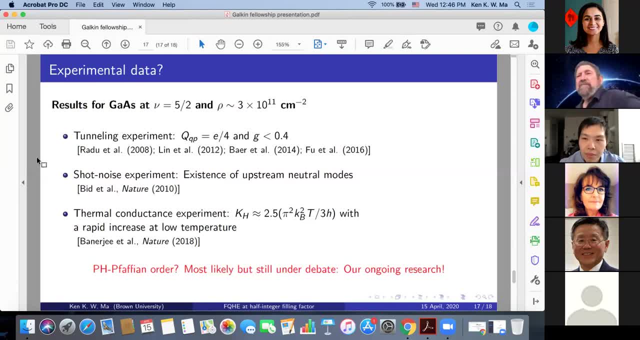 it means that if one 리�ığı o légit fait, there is no state of some value, right, Right, Correct. Remember that the end target is our rotation. the rotation of the opponent is what. But it means that we're going to sort of optimize that theбыं you know we're doing. 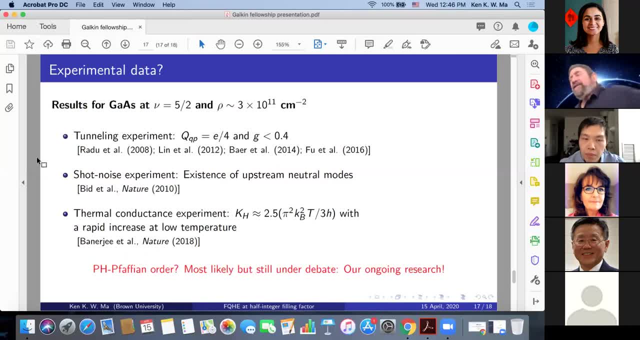 Okay, Thank you. Okay, I can go back to the one with the very first example of�딯 іê我不ł€ų Wahlq고, which calor 真的 say that this experiment says that we, that the state is this we really need. 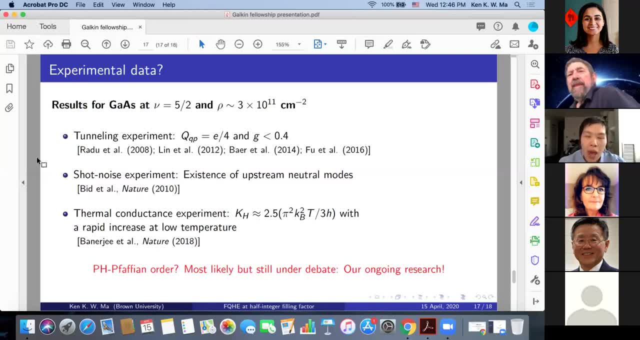 some sort of smoking gun prediction. yes, yes, yes. so actually by just measuring T or C whether there are a few neutral modes. basically, we cannot pin down more and they really to combine different experiments. but one of the experiments shows that. I mean the thermal conductance experiment shows that the 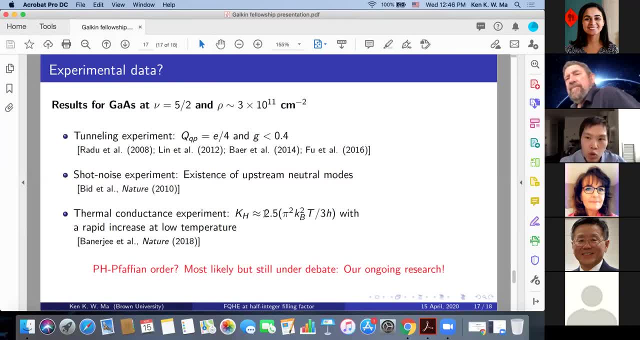 thermal home buttons is 2.5 and these 2.5 and be explained by the pH 5 an order in the most natural way. indeed, it also shows a very quick increase of thermal hall conditions at low temperature. if you combine the value of 2.5 and this rapid increase of thermal conductance, only pH 5 in order can. 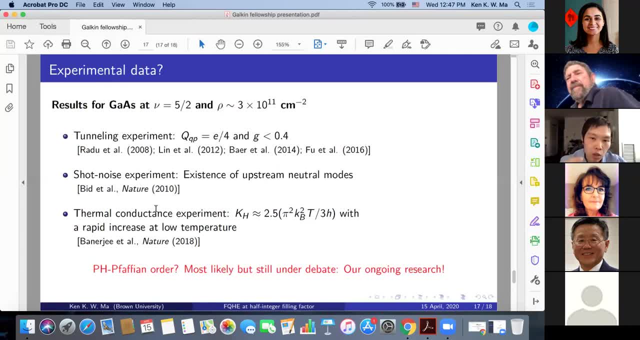 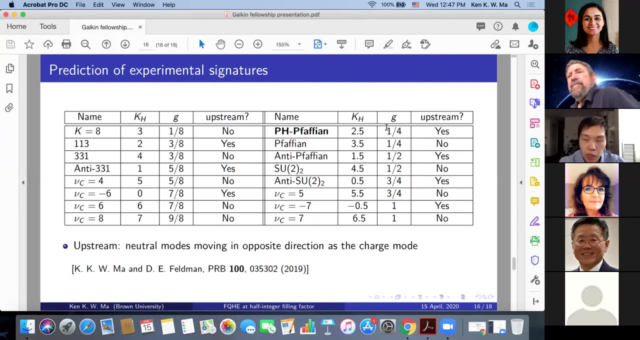 explain it in a natural way, in addition, by explaining 2.5 at the rapid increase of thermal conductance at low temperature temperature. let me go back to the previous table. GE should be smaller than 0.4 and pH 5M order is predicted to have 0.25.. This agrees, and also pH 5M order also. 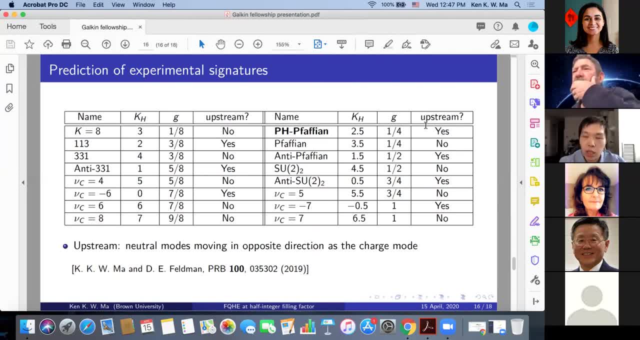 have upstream neutral mode, That's also agree with upstream neutral mode measurement. That's why, by combining these three experimental data, we are confident that pH 5M seems to be the strongest and in the most promising candidate. So you cannot just do one type of experiment, You need to do several types and then convince yourself that this topological order can agree with all experimental data in a natural way. 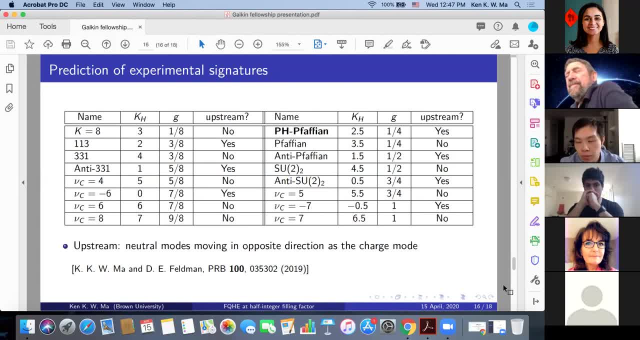 So, Mike, can I add some comment to what Ken told, Because this just reflects a rather unusual position of this five-half state in the field. The amount of experiment pointing towards pH 5M is as big or bigger than what we have in a. 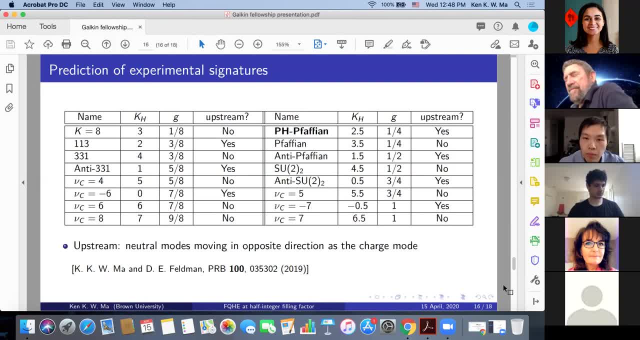 typical case For a typical quantum whole plateau. we are very confident what the topological order is. If numerics didn't exist, the problem would be considered completely solved. Of course it's pH 5M, But there is numerics. It points in a completely different direction and points there for two decades. So what's going on? 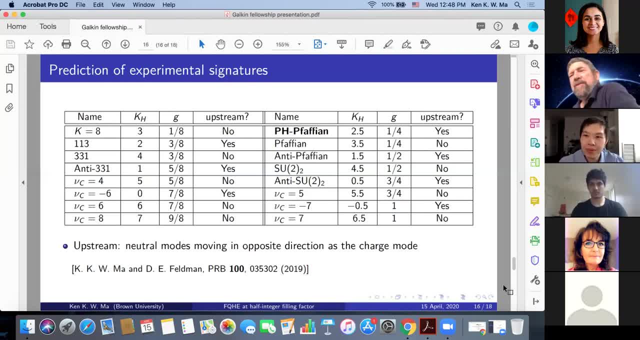 Well, isn't the numerics a little bit untrustworthy because I thought it used very, very few electrons because, simply, it's too difficult? Well, this issue is present in much of the numerical work. There are other issues And, honestly, the number of issues is very, very, very large. But, as you can imagine, very few people can do experiments. Very many people can do numerics in part because you just have it written by a certain person and everyone can run the same code and get exactly the same results. 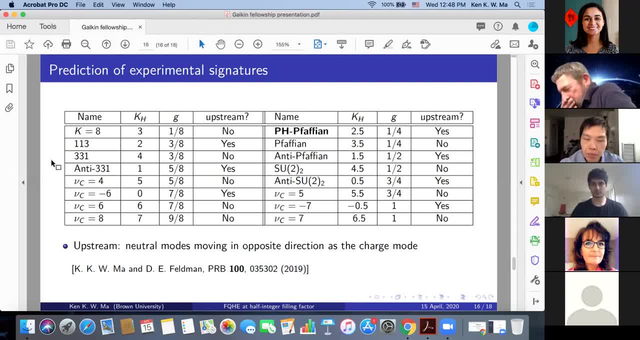 And now you have so many people invested in these being 5M or anti-5M that you've got a complicated situation Right. And I understand this, because doing a numerical investigation requires you to really, you know, throw the computer at the right bit of the problem, because the problem is, in general, much bigger than your computer can handle. So you really have to throw the computer at exactly the right bit. 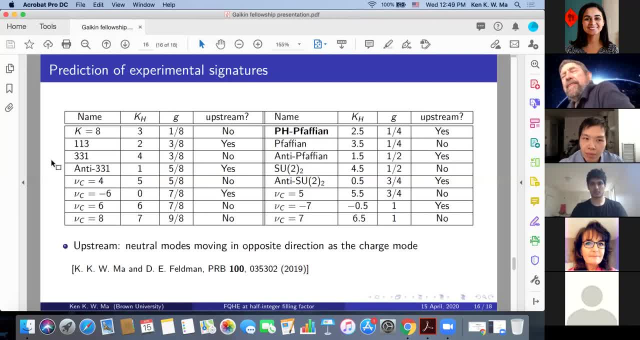 There is only one person who tries to include disorder in numerics, Donna Sheng. So she and her co-authors actually see signatures consistent with pH, But of course there are questions about what exactly she is doing with disorder, and no one else even trying. So here we are. 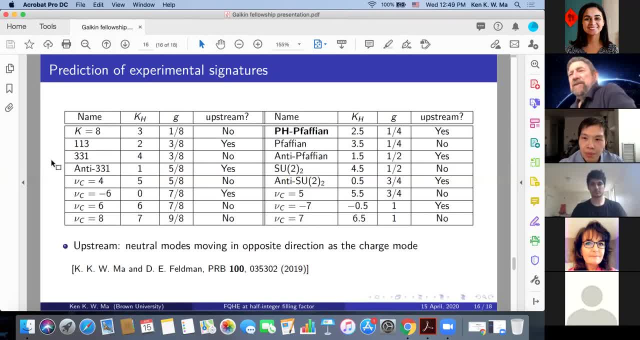 Okay, so the whole picture is a little bit up in the air still. Yeah, it's not easy, But of course the common wisdom of numerical people is that disorder doesn't matter. Given that disorder is huge, much greater than the energy gap. actually, one would think that it matters more than even the energy gap. 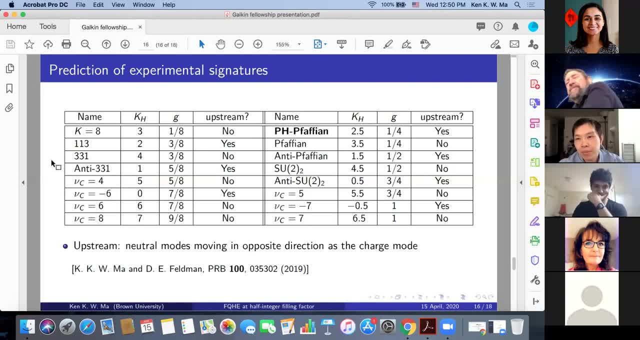 But because disorder is essentially impossible to include, And numerics the common wisdom is, it cannot matter, Otherwise what are we doing here? So you see, Yeah, right, Okay, so it's really of course, disorder is always a terrible problem. 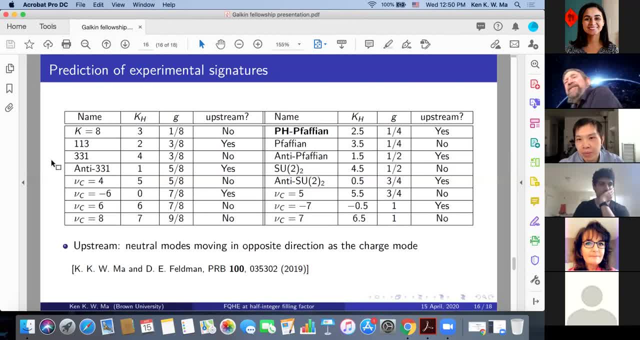 But for the quantum Hall effect you do need some disorder, so you can't do without it. Yes, without disorder you have no localization, so nothing works. But when you do, even an apparently gap state is actually compressible To some extent this issue. 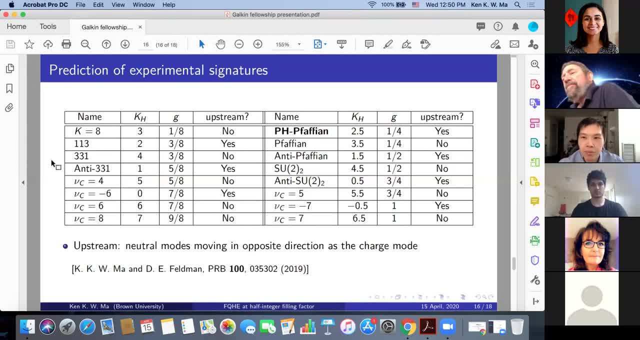 This issue is present even in integer feeling factors. If you wait long enough, you see that voltage equilibrates through your integer sample with feeling factor, say, two or three. That's a very well-known effect and many experimental techniques are actually based on that equilibration. 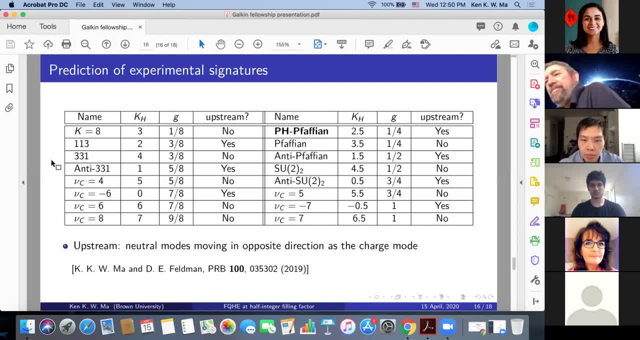 But of course canonical piece of theory and definitely any textbook would pretend that the thing is incompressible. But the truth is that the voltage equilibrates through the system, So disorder is still big enough to handle that Even an integer Hall effect. 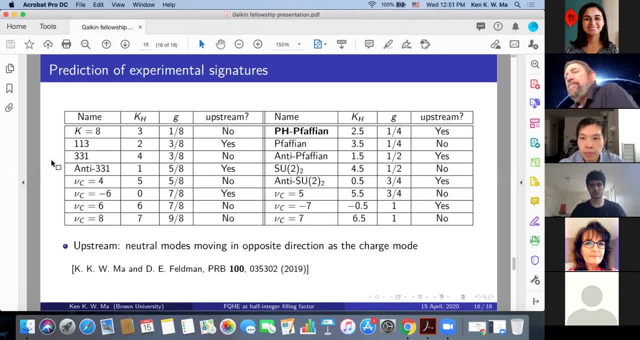 Now think of these samples. They're so fragile. One problem with numerics from the very beginning was that it predicts gaps in excess of two Kelvin And there is a single sample that shows gap of 0.6 Kelvin, typically 0.3 or less. 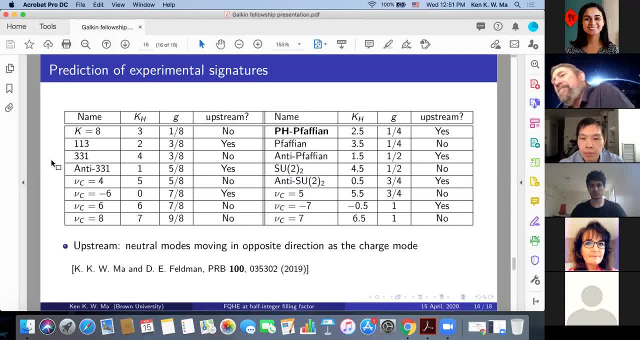 The difference is huge. At some point Morph, who is the leader of this numerical work, even wrote. even though we believe that our numerics describes these samples well, of course, a node of magnitude difference of the experimental and numerical gap is a rather big thing. 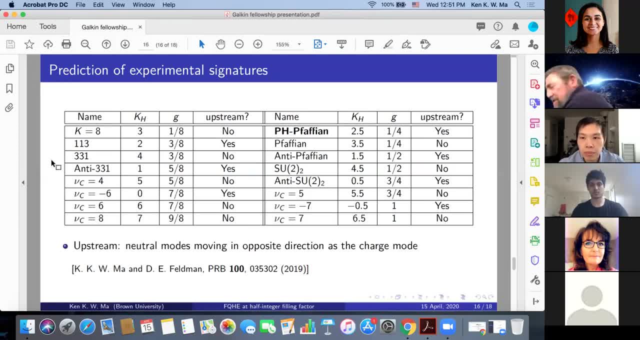 So we're not going to stretch calling this excellent agreement. yet we do So that's where we are. The gap is so bad, And the explanation actually is that disorder is so strong that, of course, it changes the gap by a node of magnitude. 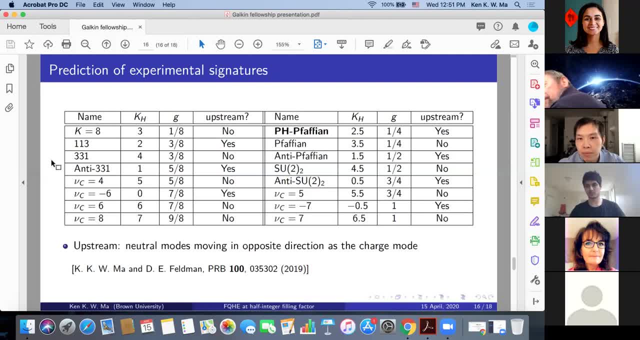 Which leads to a question: Can it do other things, like changing the topological order? That's where we came from with Philip Zucker several years ago. Well, yeah, of course. if your perturbations are big enough, of course the order can change. but 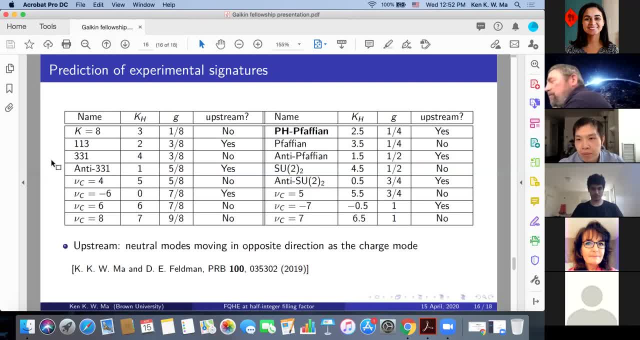 The problem is it's not a perturbation. Estimates- No, no, no, let me Disorder- shows that it's actually bigger than the energy gap. So, in a sense, quantum Hall effects is perturbation on top of the disorder, not the other way around. 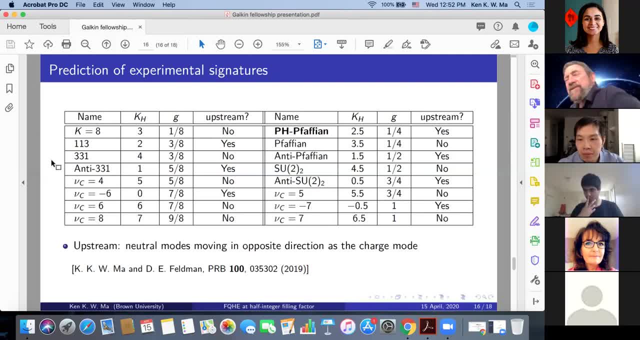 Right Now I understand what you're saying, But I mean. what I was meaning was that you have your ideal theoretical system and your real system has got some deviations from that which I'm calling perturbations, regardless of how big those deviations are. 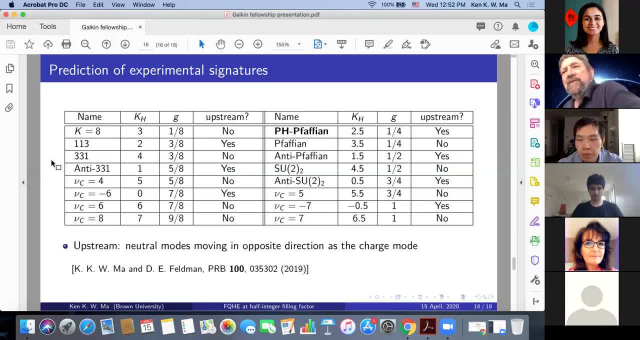 And so your physical system differs considerably from your ideal theoretical system, right, Dima? Yes, Could we give Quok a chance to answer the question? Oh, I'm sorry. We had such a heated discussion with Mike. I'm sorry. 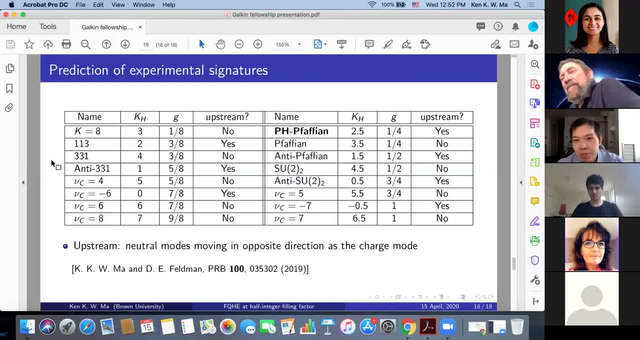 And then see whether there are other attendees who have questions. Hi Ken, Thank you for the talk. I just had a question, actually, about this slide. Could you speak a little bit more to the methods that you use to get these values for the different options? 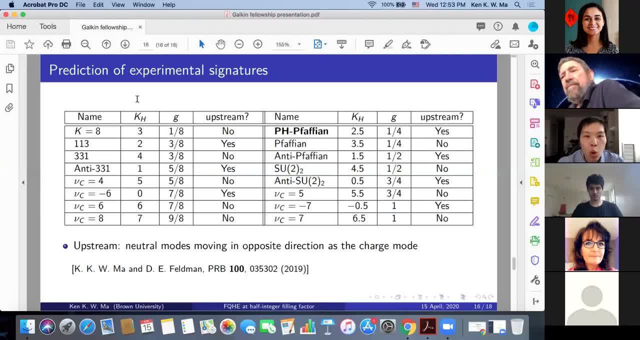 You mean this one, Mm-hmm. Okay, So for the thermal Hall conductances, what we do is like: So the S structure out, and then, because this table is for the five half-states, so I must have two integer modes, and then they will give two to these thermal Hall conductances. 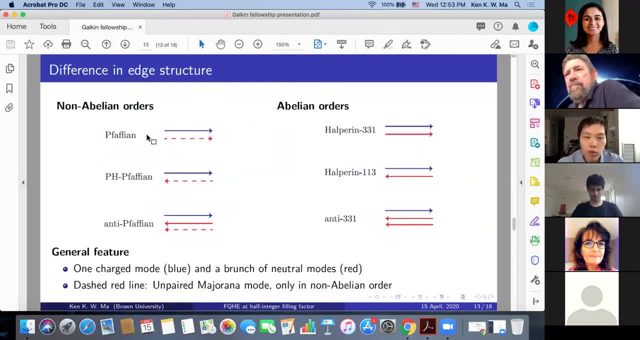 And then I need to go back. let's say here For the 5 here I will have an additional charge mode here and then a red dash right to the right, So I will get another 1.5, so I will predict 3.5 for 5 here. 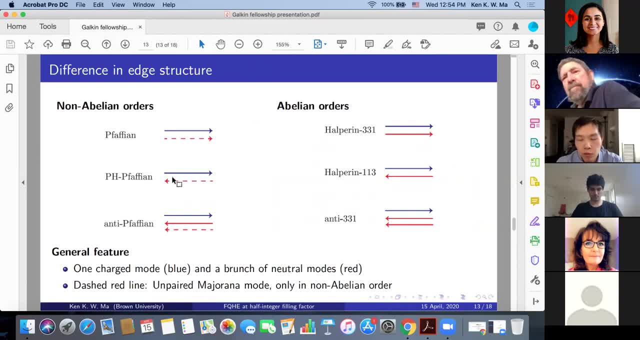 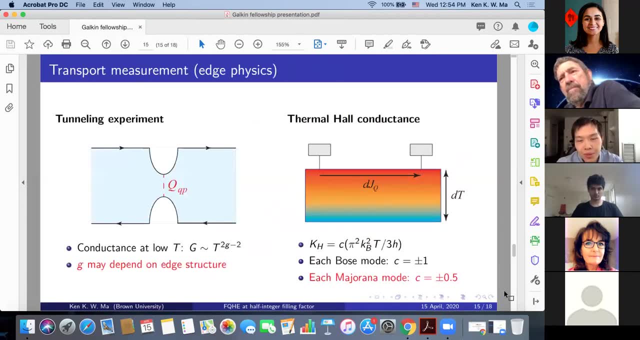 And then for pH 5, here I will predict 2.5, something like that, If you are talking about thermal Hall conductances. and then Erin, what's your question about what technical methods he is using? Yeah, I suppose. 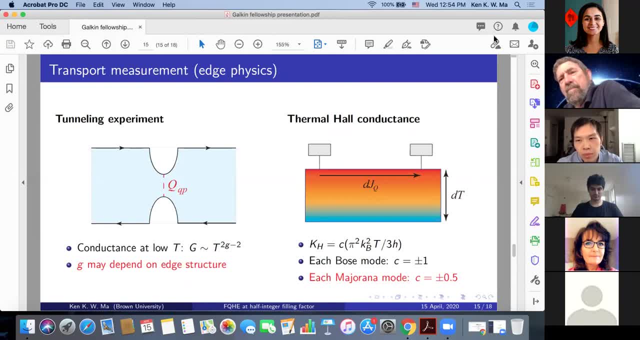 I guess I understand the theory that goes behind those numbers, but I didn't know if it was more of a numeric question. It's a form of theory and quite a few other things. So I think you're answering the wrong question. What are the technical tools you're using? 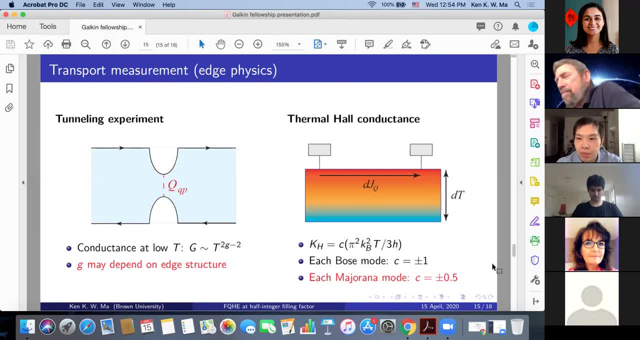 It's more like conformal theory, But many other things, right. What else? Yeah, like leaking long, So like in the liquid theory, and then yeah, something like that. yeah, Okay, thank you, You use the technique for interferometer, all sorts of things right. 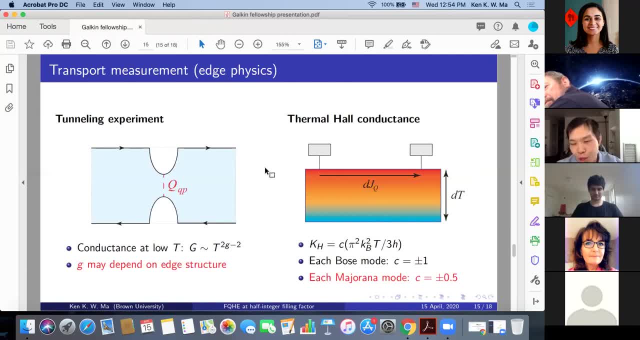 Yes, but yes, in principle. yes, But in real situation we don't really use those advanced at least. But if you are talking about the underlying principle, yes, Okay, Any other questions? So can I ask a very difficult question? 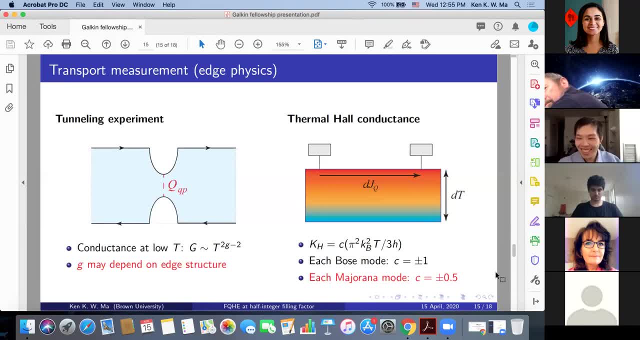 I know I'm an advisor, Maybe I'm not supposed to, But I want to ask your thoughts about graphene Because obviously at Brown our best chance to probe half-integer physics is in graphene. And what do you think would change and what would stay the same compared to gallium arsenide? 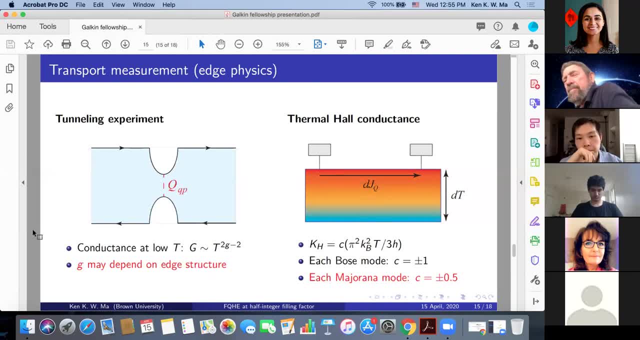 So, first of all, first of all, we know that in graphene the energy dispersion of the electrons, which is I mean those electrons you know are responsible for quantum ball, are quite different, as in gallium arsenide. In gallium arsenide, at least, the first thing I can tell you is: 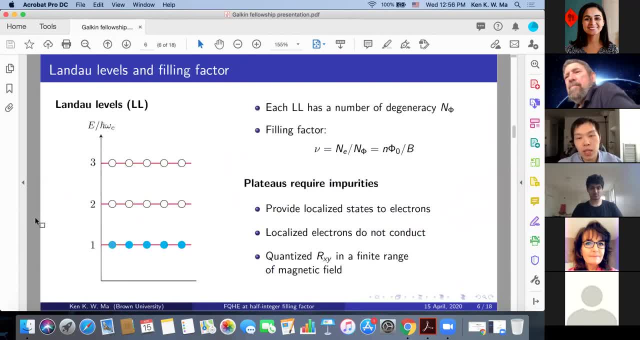 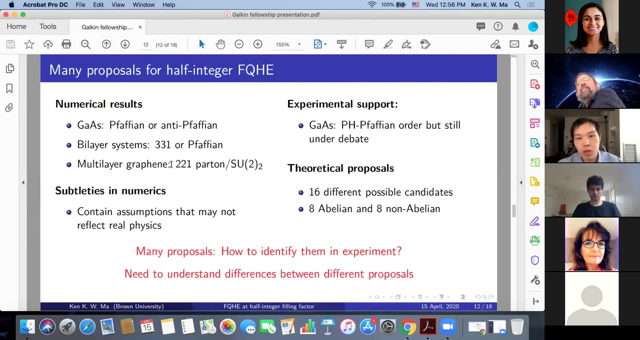 the Landau levels will not be equally spaced in graphene. And then if you are talking about half-integer quantum ball state in graphene, then the only thing I know let's say in multi-layer graphene, then I will. their prediction is another topological order. 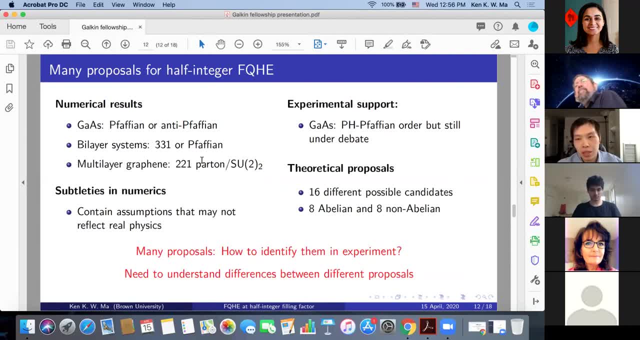 In fact in bilayer graphene there's also a debate on whether 331 or D321 parkon, But it seems that the farbium or the antifarbium order, I don't. I don't think there are many studies which support these two in multi-layer graphene. But if you are talking about monolayer graphene, then at this moment I cannot remember which candidate is more promising there. But I wonder what happens. cannot be that this state and anti-this state are equally likely, as often happens in, and then disorder will naturally mix them and produce their average? 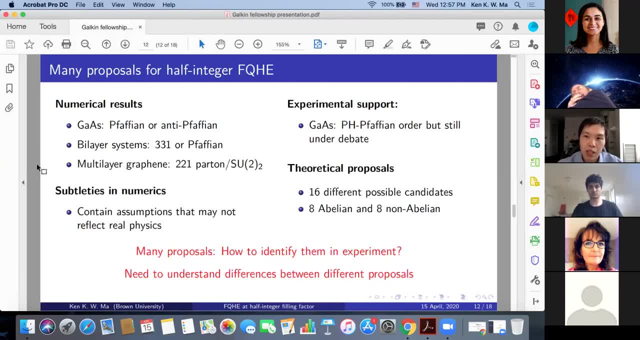 which is again pH 5.. Yes, yes, yes. And let's say, if you are just perfectly half-built, there should be an exact particle-hole symmetry there, But there is no exact particle-hole symmetry in gallium arsenide. 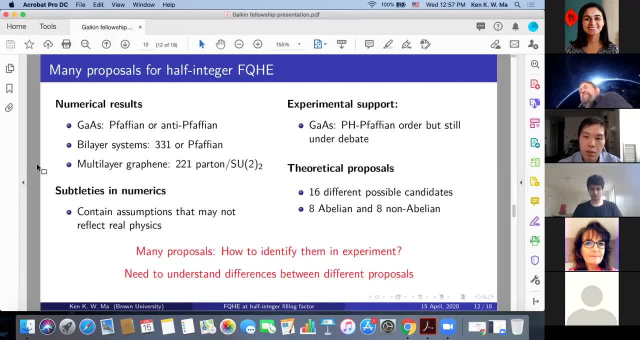 That's another miracle. Yes, yes, yes. But as you mentioned, there may be some impurity effects also in graphene, and this impurity effect may be very important there, because you already keep the light away from the choice point there. 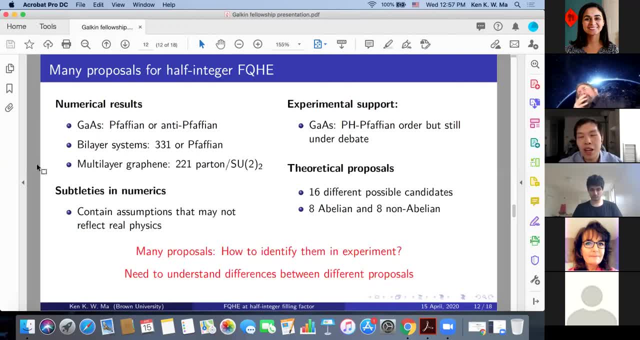 So I don't know, Yeah, I don't have. I don't have a good answer to which candidate is more convincing there. And I think there is thermal hole conduction experimental data in graphene, but not yet for half-individual quantum processing in graphene. 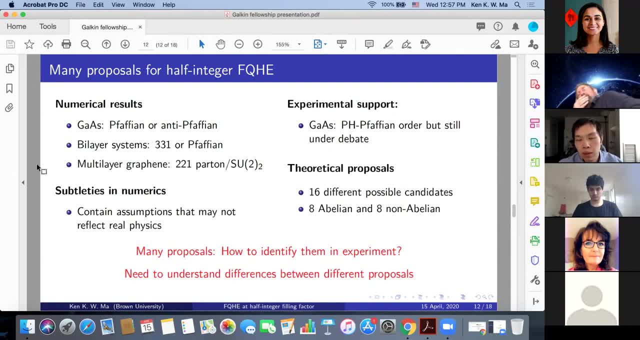 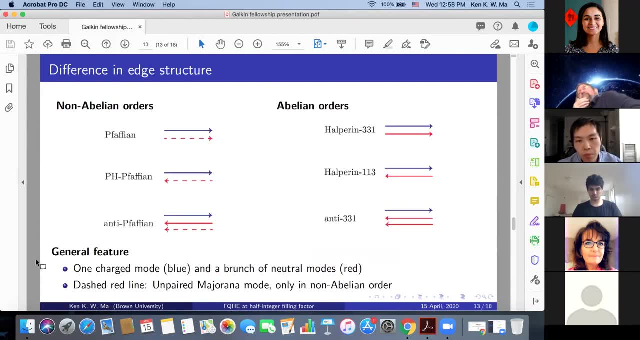